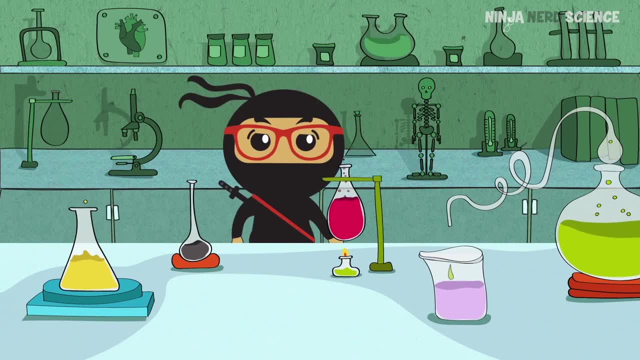 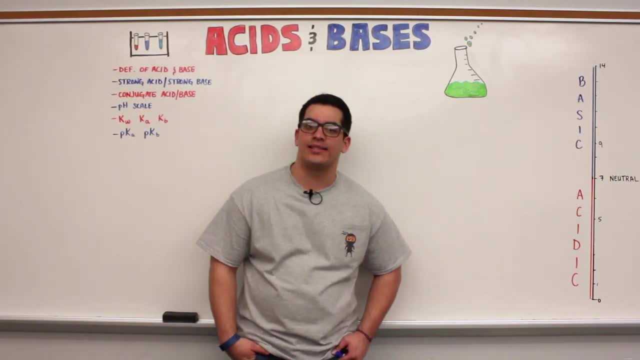 All right, Ninja Nerds. So what we're going to do in this video is we're going to talk about acids and bases, So we're going to go through first off before we get into any calculations, because that's what we're going to spend a lot of time on, Kind of the key to chemistry and getting better at. 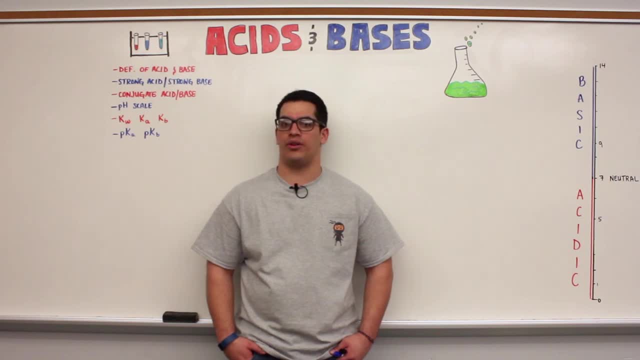 it is doing tons and tons of practice problems, And so that's our goal. What we're going to do here at Ninja Nerd Science is help you as much as we can with a lot of practice problems. Before we dive in, let's go ahead and get some just baseline introduction, introductory material out. 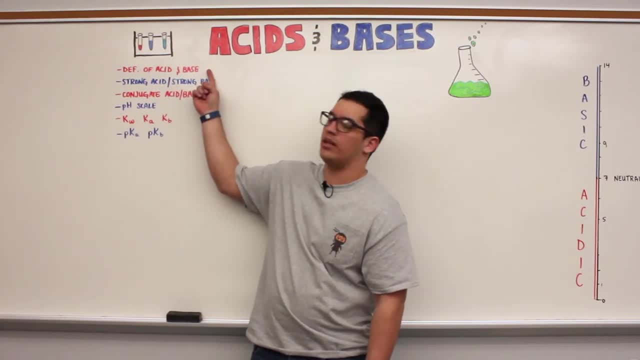 of the way. So first off, let's go ahead and define what an acid and what a base is All right, So we're going to do that. Then we're going to talk about all the strong acids and strong base We're. 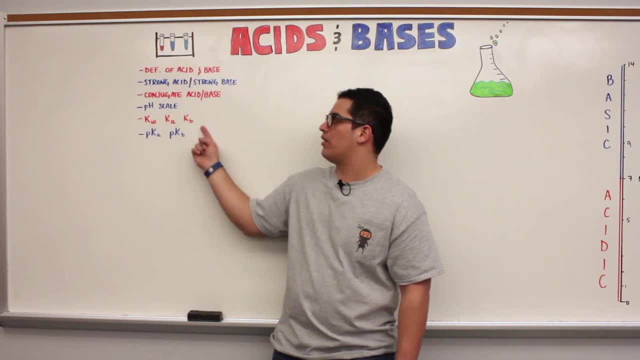 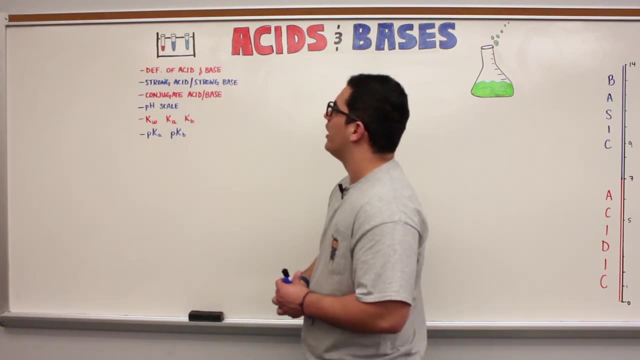 going to talk about conjugate acid, conjugate base, pH scale, And we're going to talk about this: KW, KAKB, PK, PKB. All right, So let's go ahead and dive in first with the definition of an acid and a base. In order for us to do this, though, we have to go through three different 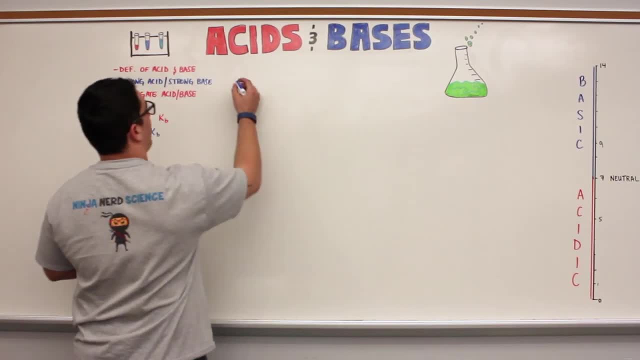 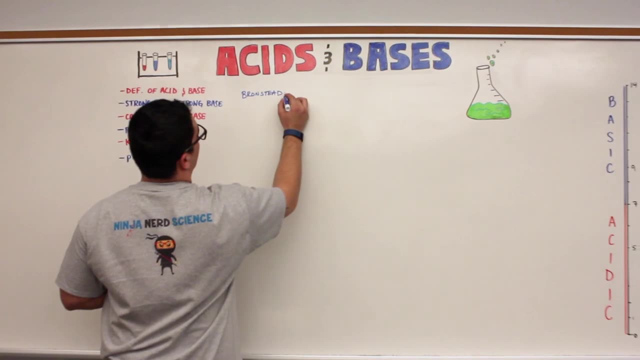 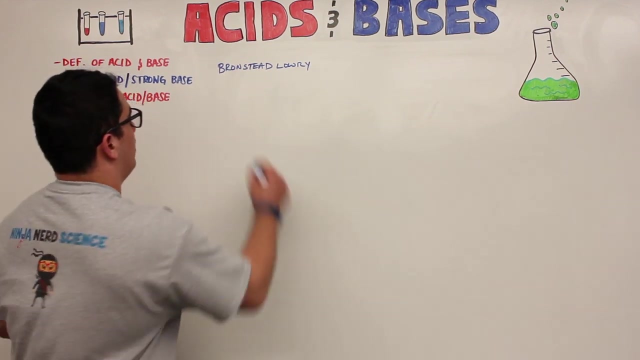 types of definitions, All right, So the first one we're going to talk about is Bronsted-Lowry. Okay, So Bronsted-Lowry, So Bronsted-Lowry acid. And when we're talking about a Bronsted-Lowry acid, he said that when you take an acid and you 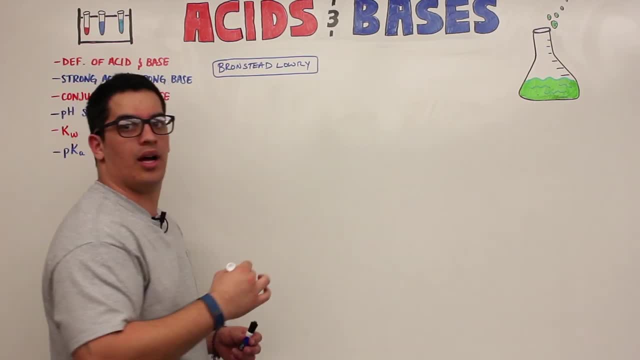 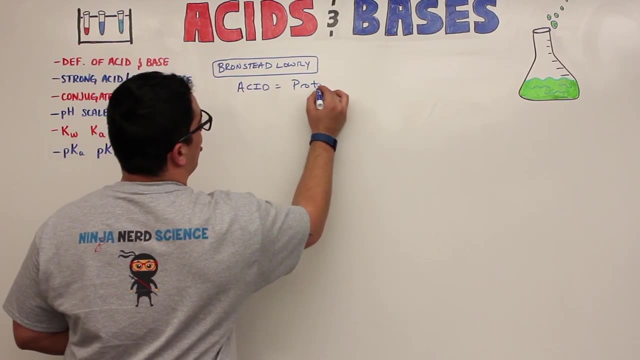 put it into a solution: an acid gives up protons. So how does he define an acid? He defines an acid as a proton donator. Okay, So he defines an acid as a proton donator. Okay, So he defines an acid. 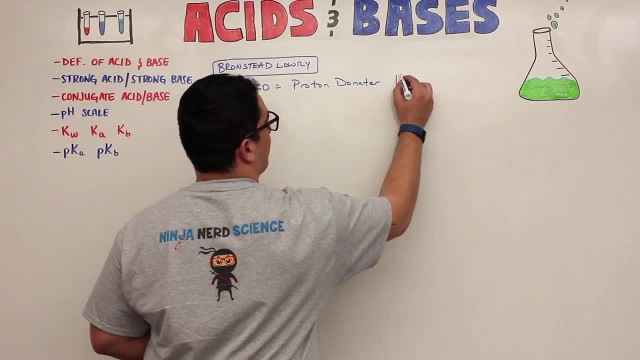 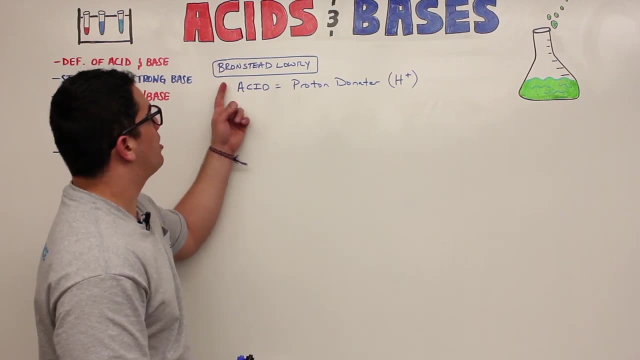 as a proton donator, Okay. Or we can even draw this like this: He loves to give up H plus ions, because we're going to see this a lot, Okay, Whenever we're doing a lot of these practice problems. So again, what is a Bronsted-Lowry acid? by definition, A proton donator, Well. 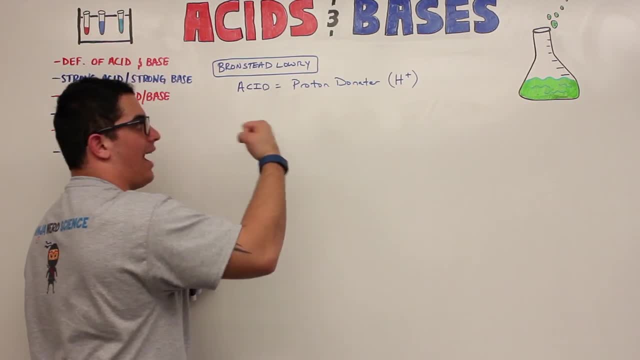 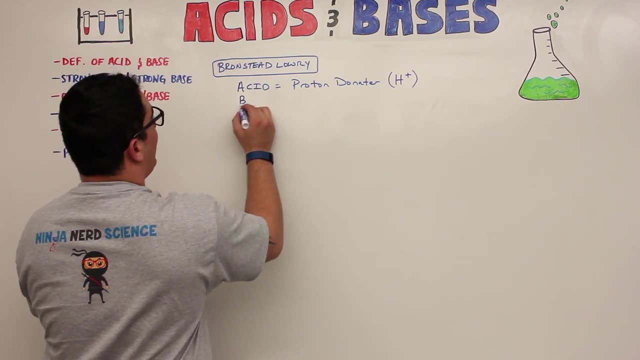 if an acid is a proton donator, someone has to be able to gain that or accept that proton. Who accepts the proton? The Bronsted-Lowry base. So the Bronsted-Lowry base is going to be the guy who is accepting the proton. So he's going to be the guy who is accepting the proton. So he's going. 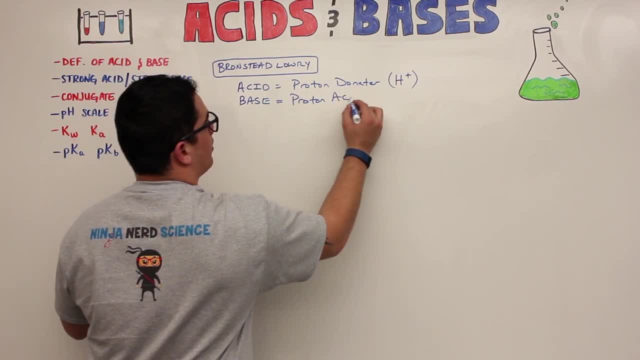 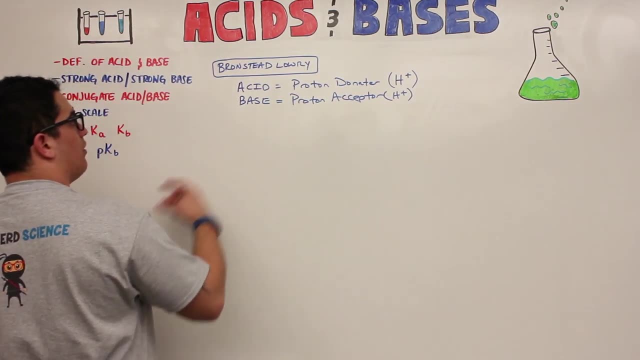 to use a proton acceptor. All right, So that's pretty easy, right? So it's not too bad there. So, for example, if I were to ask you if I were to draw, right here, let's say I did this- H A plus. 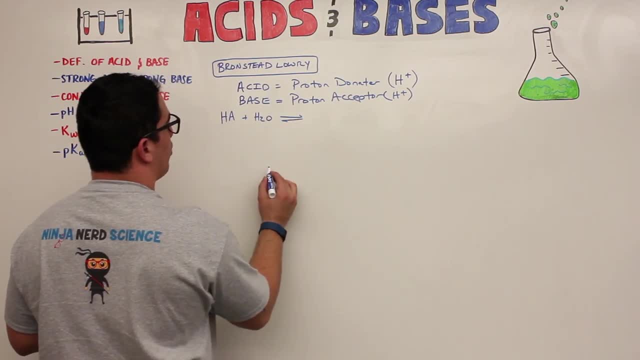 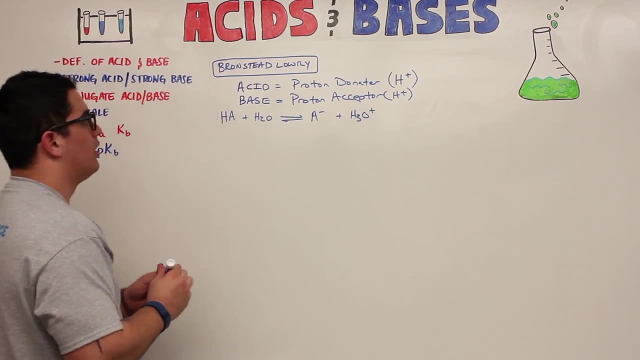 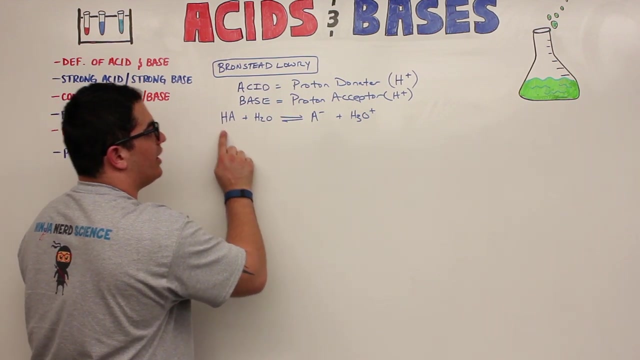 water and it yields two products. Let's say one of them is a negative and the other one is H 3 O plus. If we were to go based on this definition of Bronsted Lowry, what happened to this H A? It turned into a negative. So what did it do? It gave up a proton. 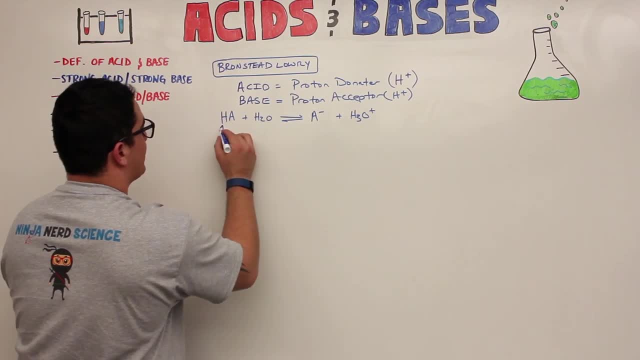 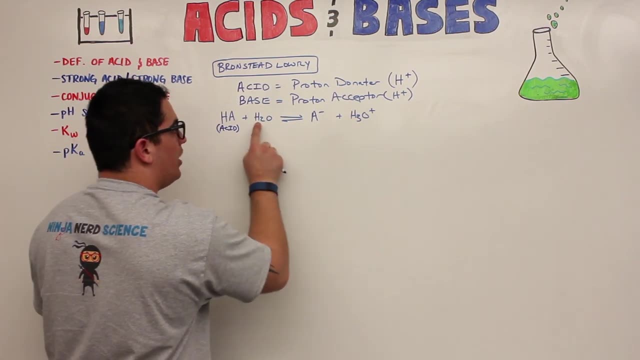 So he must be, by definition, the Bronsted-Lowry acid. And then what happened to this H 2 O? He turned into H 3 O plus hydronium. So he must have accepted that proton. And if he accepted the 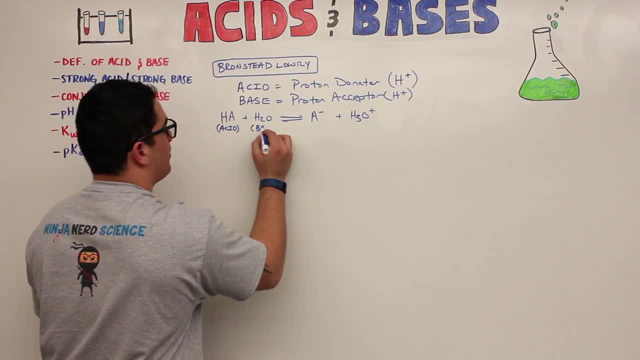 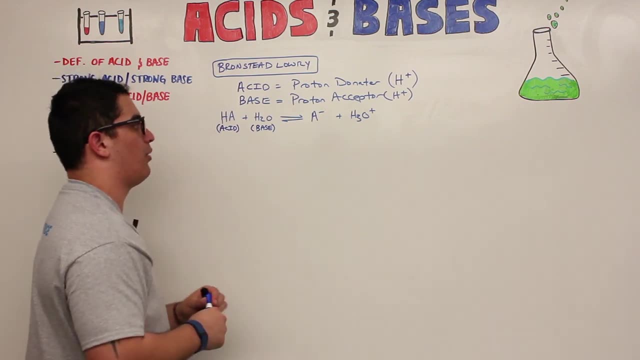 proton that the H A gave, he must be the base. Now, while we're here, let's just go ahead and get these terms out of the way, Since we're already here: conjugate acid, conjugate base- Those terms out of the way because we're already here. So, an acid when he gives up the proton. 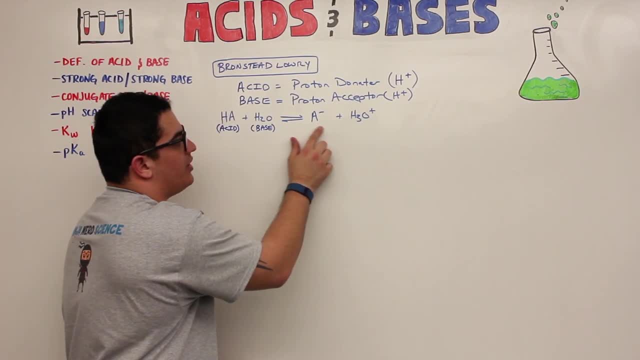 so he donated that proton to the H 2 O. he turns into a different term now that we can call So he was an acid, but now he's a base By definition. if he's a base, usually bases have negative charges, right, So they're really good at having negative charges. That's kind of the way that we 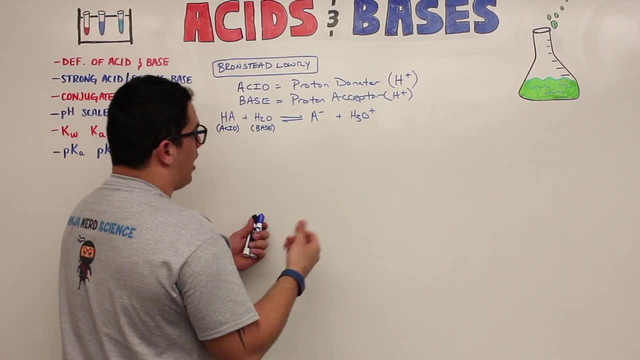 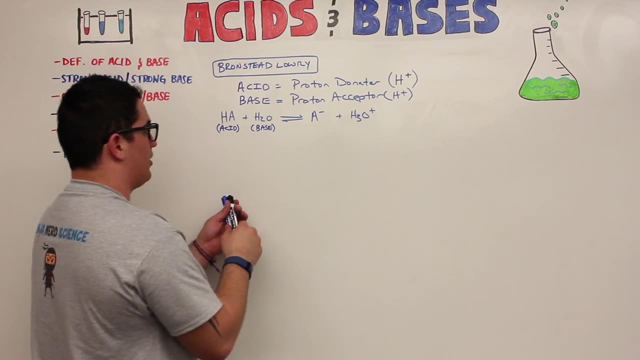 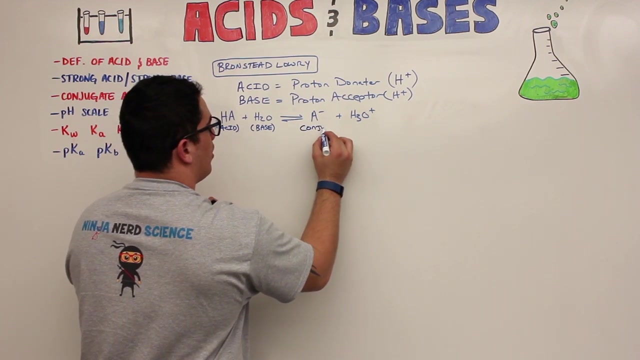 can see bases is they're negatively charged molecules or atoms. So we're going to say that this is a type of base. It's the conjugate base. So this acid, it gets converted into a negative, which we're going to call the conjugate base. And again, why is he the conjugate base? Because the 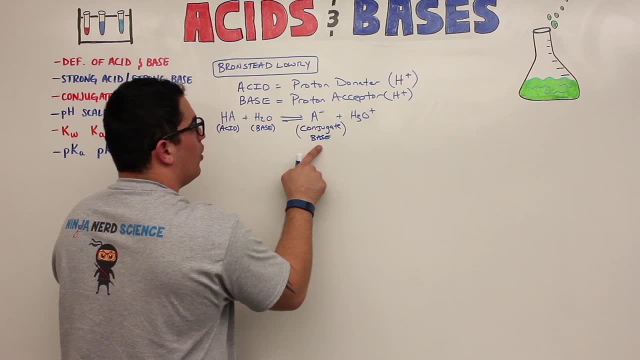 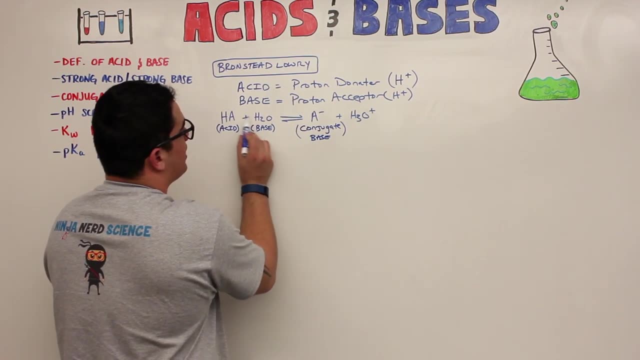 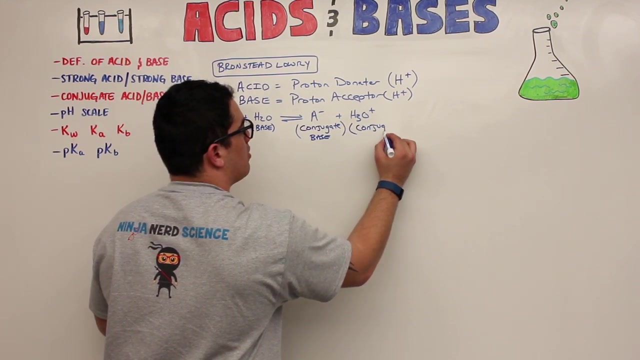 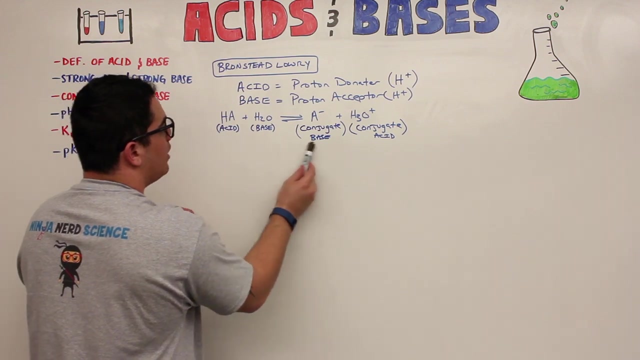 acid gives up a proton and turns into a conjugate base. Well, if he turns into the conjugate base, then this must be the acid. Why is he the acid? Because this water when he accepts that proton. so he is the conjugate acid. So if we were to combine the pairs, this acid and this conjugate, 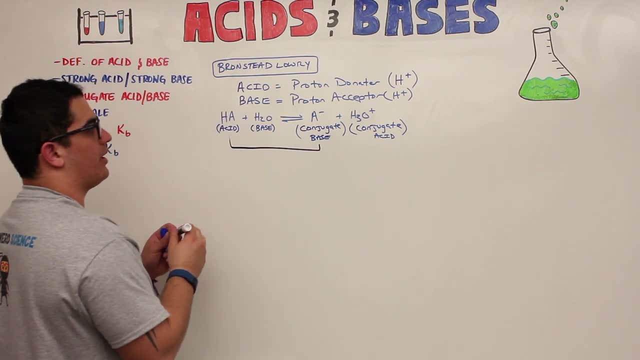 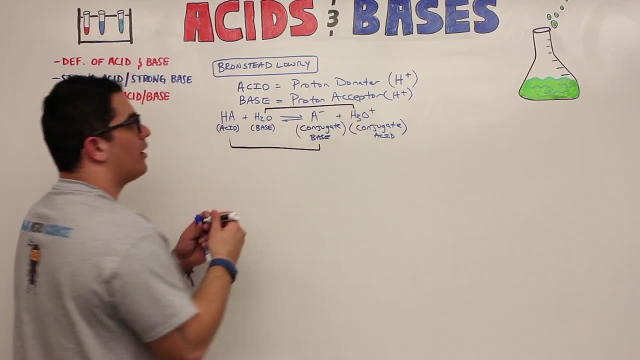 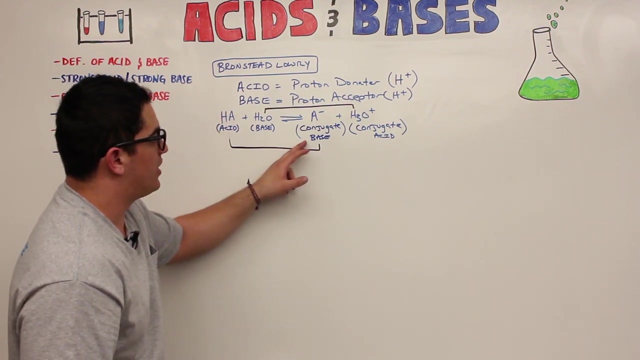 base. this is the acid conjugate base pair right there. And this right here is the base conjugate acid pair here. Okay, So not too bad there, right? So that's just giving you an understanding of Bronsted-Lowry- what an acid and what a base is. And then, what is an acid? What is its conjugate? 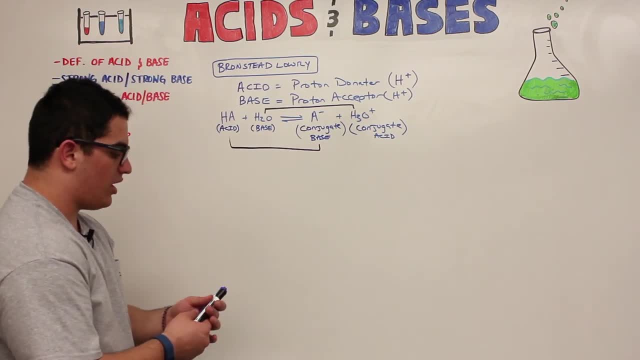 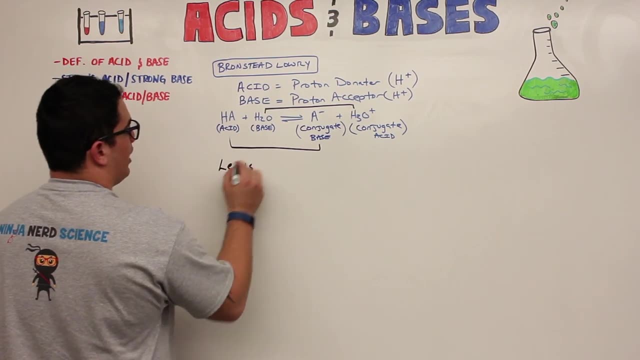 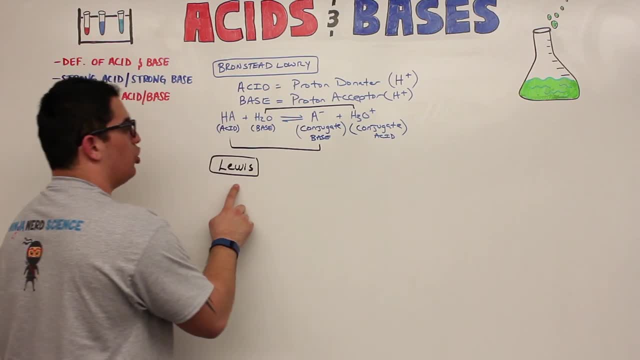 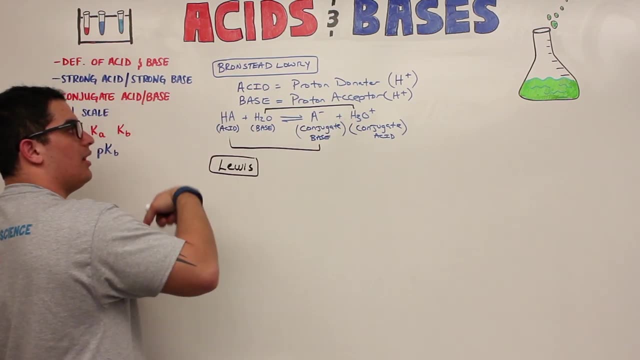 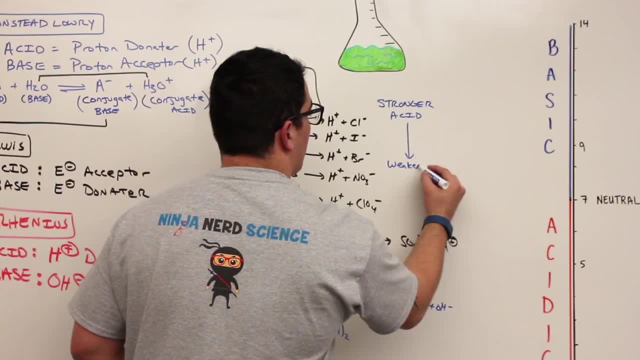 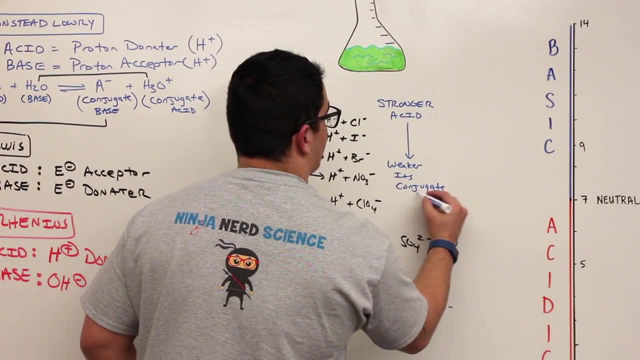 acid is a proton that accepts electrons. That's his definition. He says, by definition, a Lewis the weaker its conjugate base, The weaker its conjugate base. And this would be the vice versa: if you start off with a strong base, the weaker. 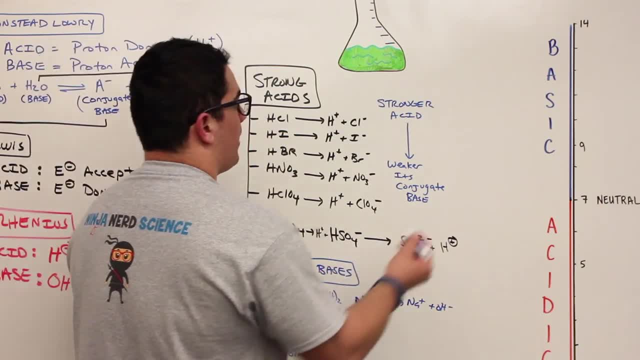 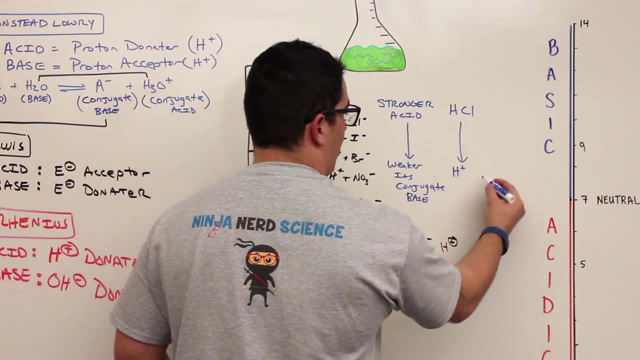 its conjugate acid. It's either way. Let me give you an example here. If I take something like HCl, I react this in water. what would I get? I would get H+, which is a strong acid, and I would get chloride. Well, this, by definition, is a strong acid. 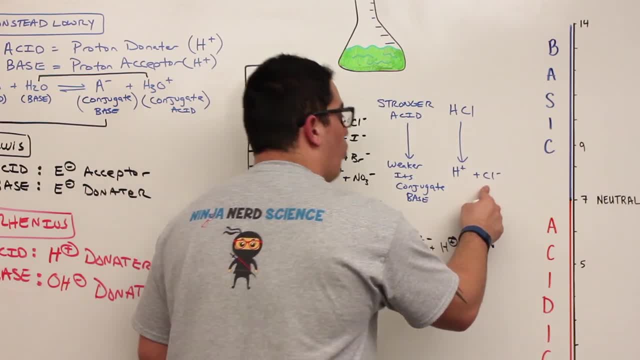 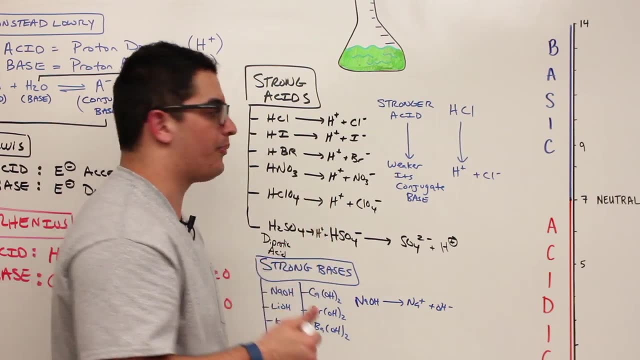 This right here is a very, very weak conjugate base. That's going to be important whenever we talk about the acidity and basicity of salts. okay, Alright, so again, remember that relationship: Stronger the acid, the weaker its conjugate base. And, like I said, you can do the same thing with the 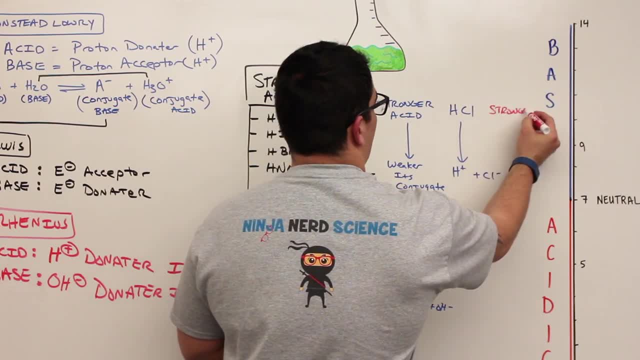 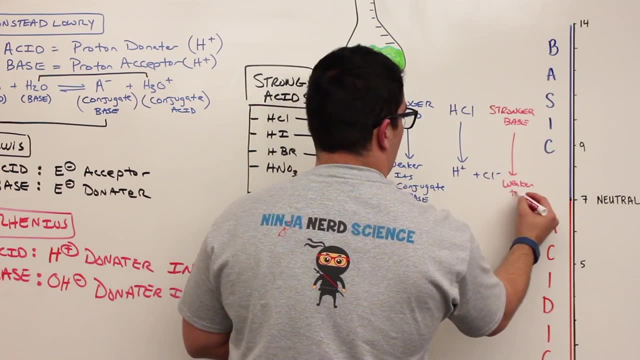 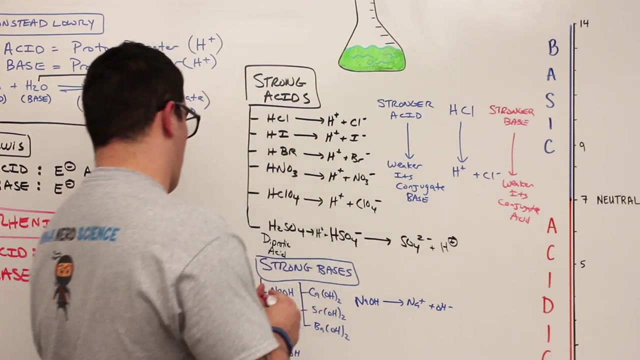 other one. You could say: stronger the base, the weaker its conjugate acid. Okay, so now we have that relationship taken care of. So what have we done so far? We've talked about definitions of acids and bases with Bronsted, Lewis and Arrhenius. 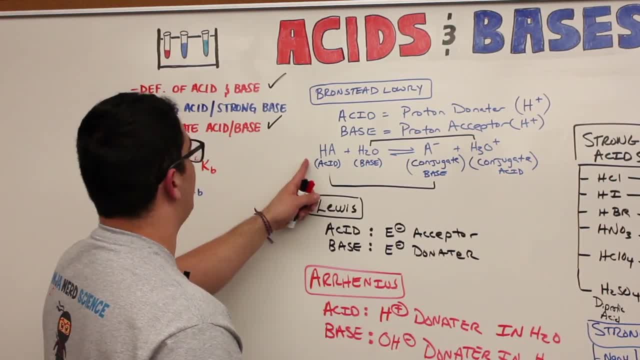 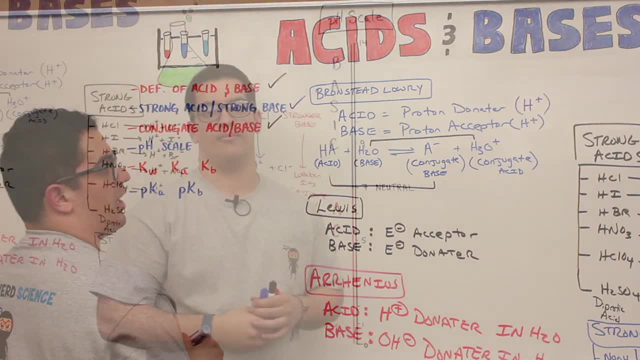 We talked about all the strong acids and strong bases and we tied in the relationship with conjugate acid, conjugate bases and the relationship of strength. Alright, let's get over here to the pH scale, Alright, so let's go ahead and talk about. 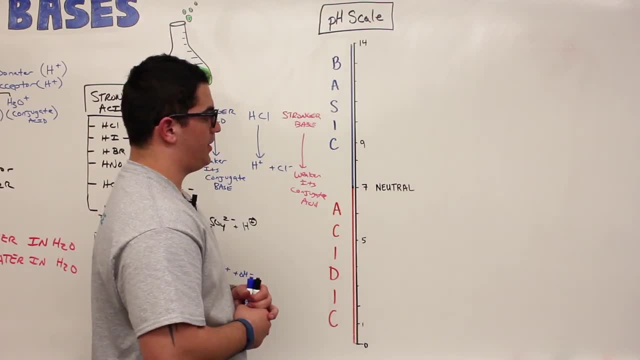 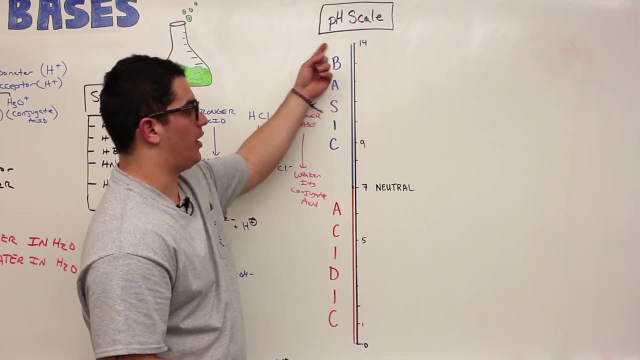 pH scale. So pH scale is basically a logarithmic scale here, and we're going to talk about that in a little bit, but just know that it's a scale that goes from 0 all the way to 14.. And what it does is it helps to measure from 0 all the way to 7,. 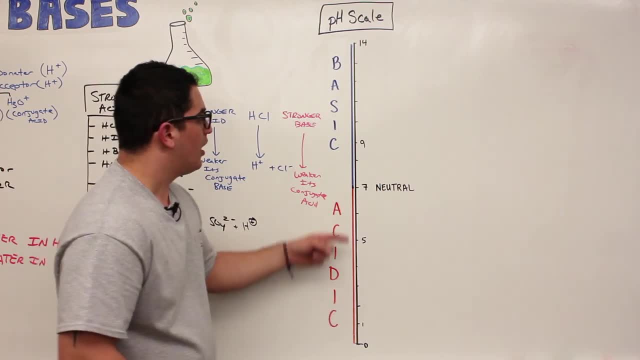 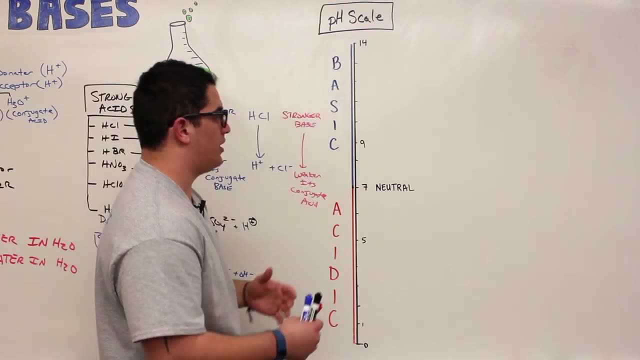 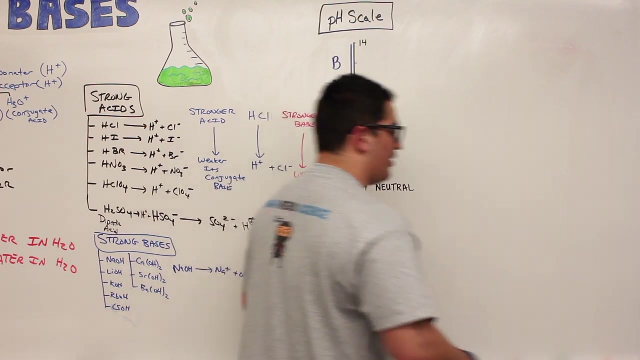 measures how acidic the solution is, And then going from 7 all the way up to 14 measures how basic a solution is. Now again, what do I mean by acidic and what do I mean by basic? So when we talk about acidic, we're talking about specifically, we're talking 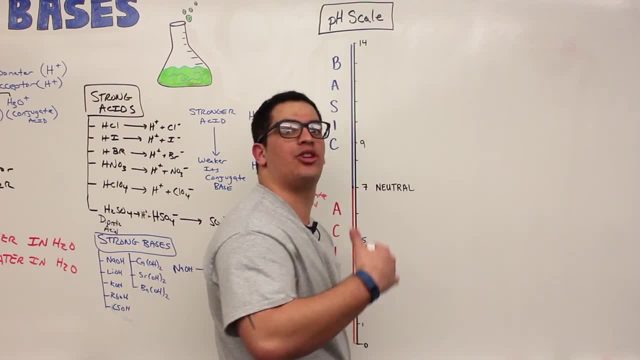 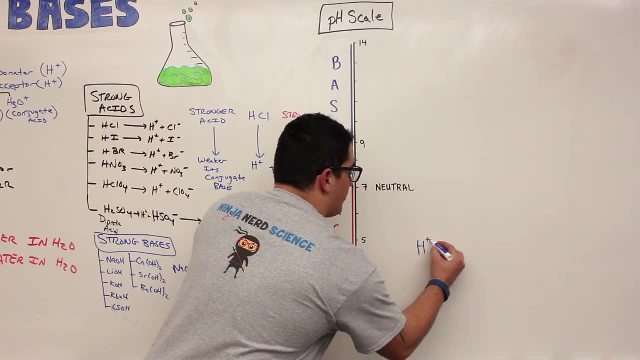 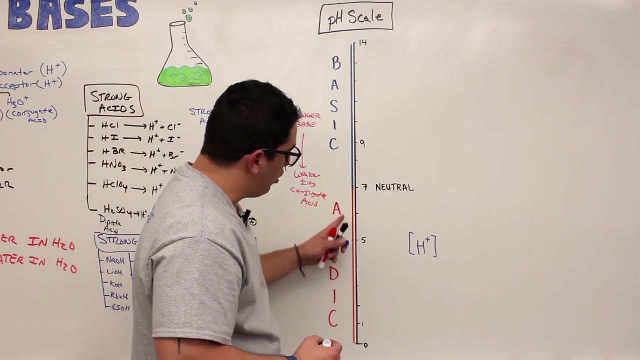 about how many protons we have or how many hydronium ions we have. So again, we talk about acidic environments, we're talking about the concentration of H plus and we put these brackets in there to signify concentration. So the more you go closer, 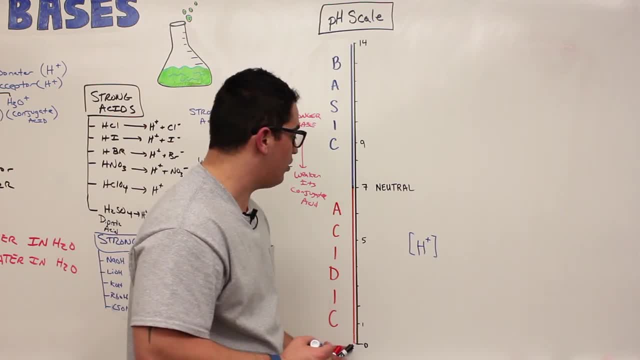 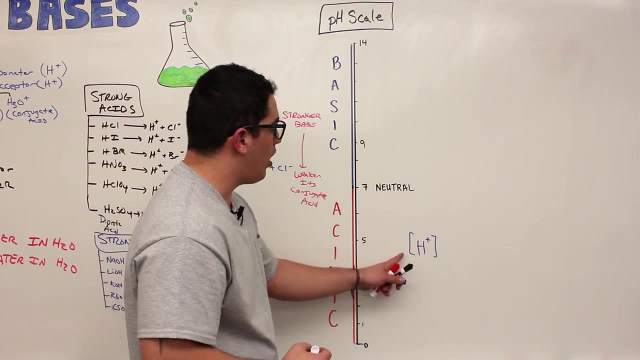 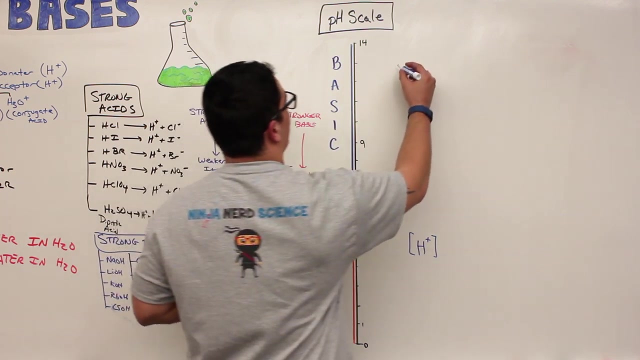 to zero, the more acidic your solution is. So if you have a solution of that's in between one and zero, that's that's pretty freaking acidic, Alright. so when we talk about acidity, we're talking about H plus concentration. When we're talking about basicity, we're talking about hydroxide ion concentration. So 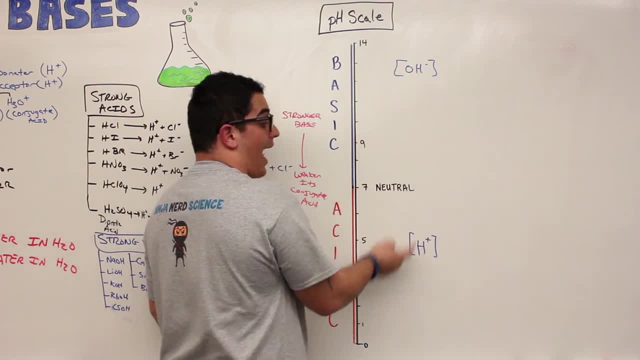 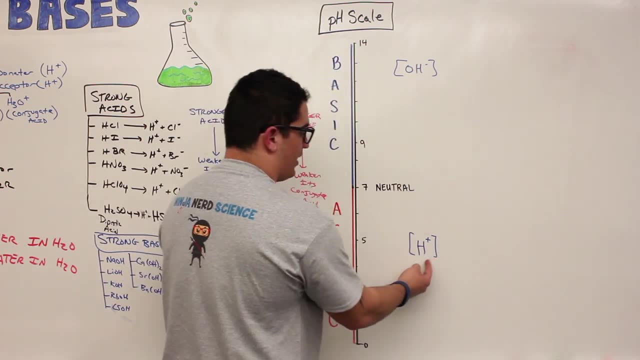 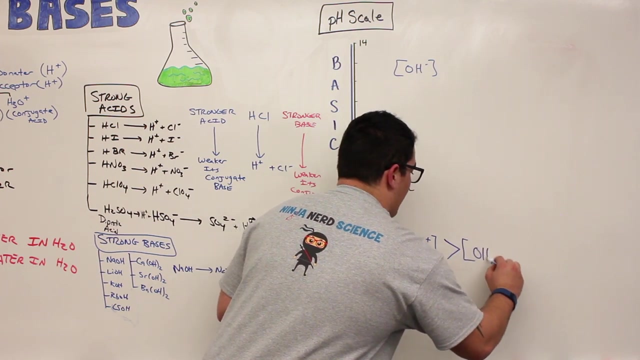 again if I were to say: okay, I got a solution that can have H pluses and I got solution that can have hydroxides. How do I know specifically that it's acidic? Well, that means that the H plus concentration in the acidic environment is greater than the concentration of the hydroxide ions. Alright, specifically in: 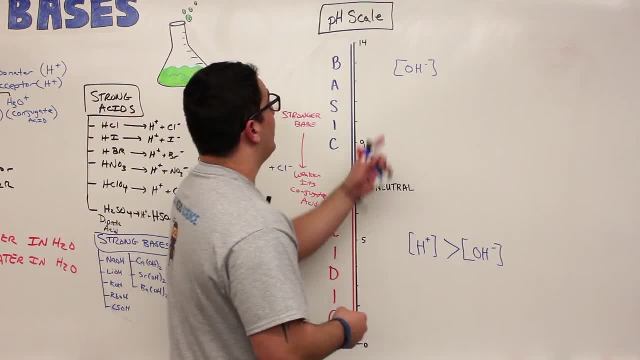 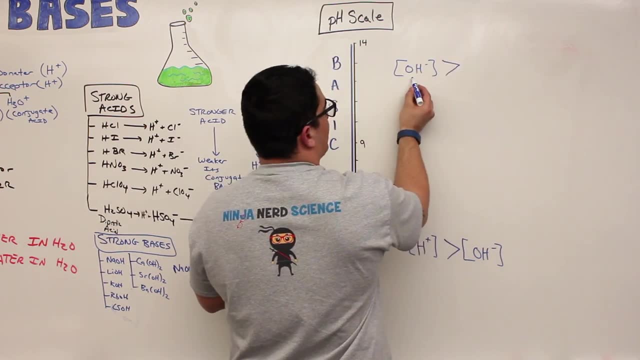 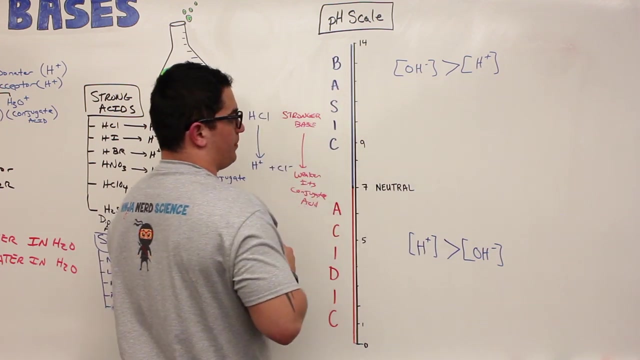 the acidic environment, Because the more H plus is, the more acidic In the basic solution- the basic solution- we want it to be measured by hydroxide ion concentration. So the greater the hydroxide ion concentration is then the H plus concentration. that means that we're in a basic solution. What if it's neutral, though? Then these: 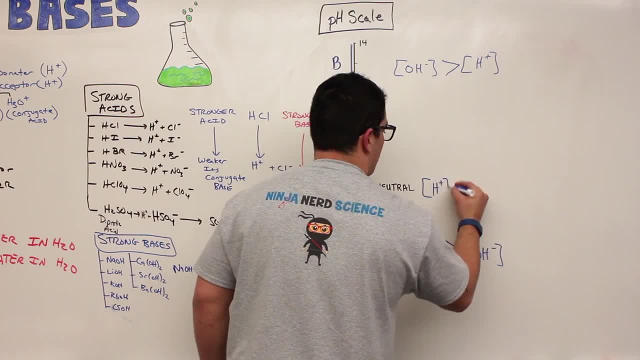 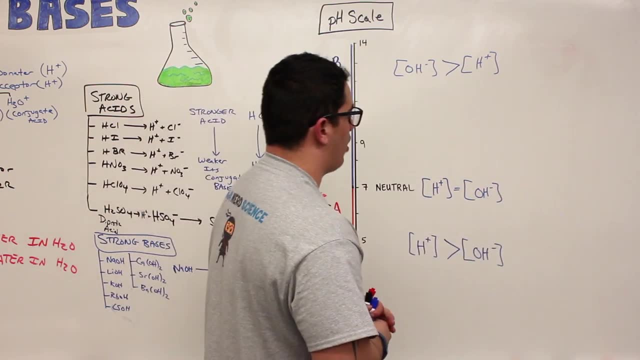 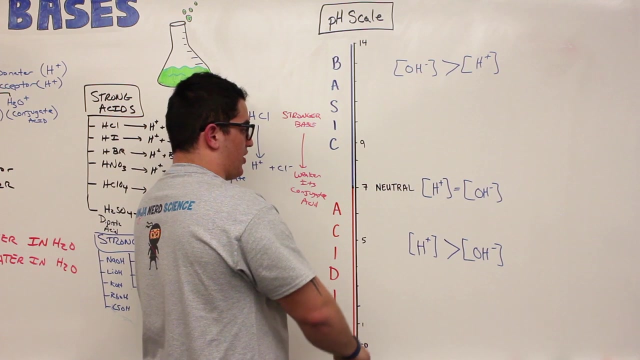 two are equal. So then the H plus concentration is equal to the hydroxide ion concentration, And this is an important relationship when we're talking about KW here in a second. Okay, before we do that, I want to talk about another thing. So I said before that this is a logarithmic scale, right? So in other 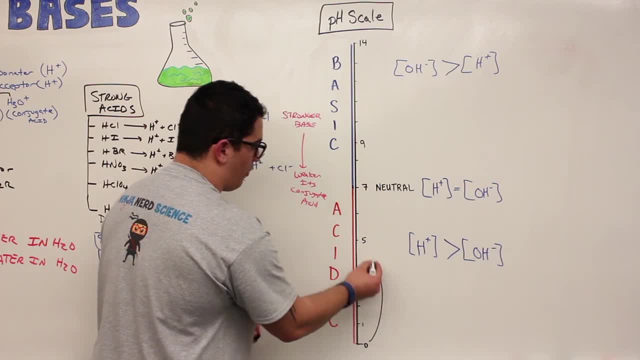 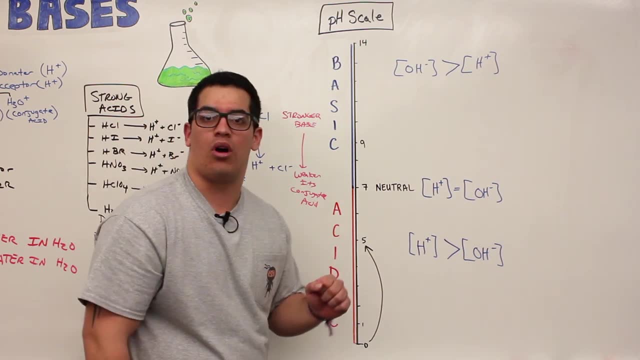 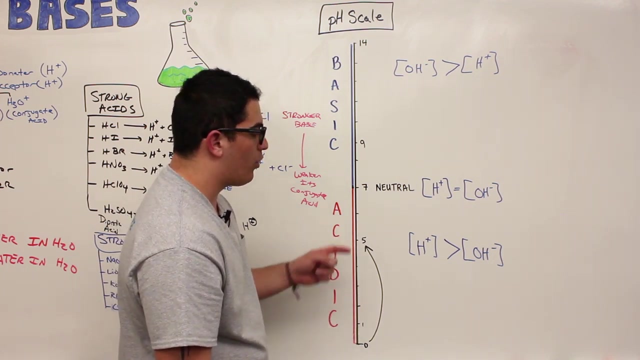 words. if I wanted to go from 0 all the way to 5, most people would say: okay, how many people was the pH change? Well, they'd be like, oh, it was 5.. That's wrong, And the reason why is each number you go up from 0 to 1,, 1 to 2,, 3 to 4, and then 4 to 5 is a 10 times. 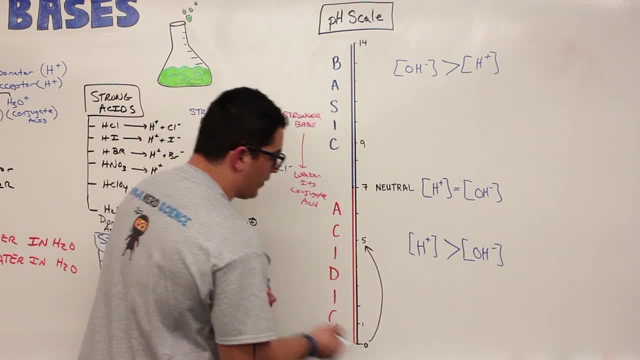 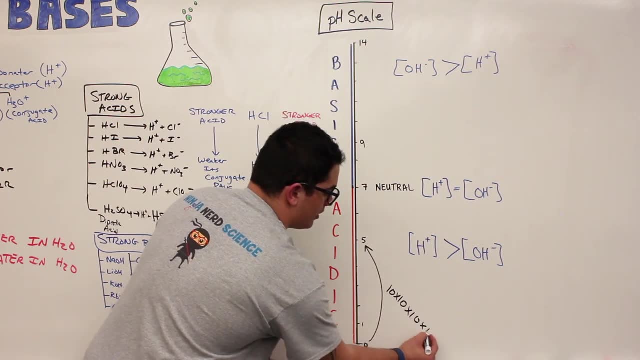 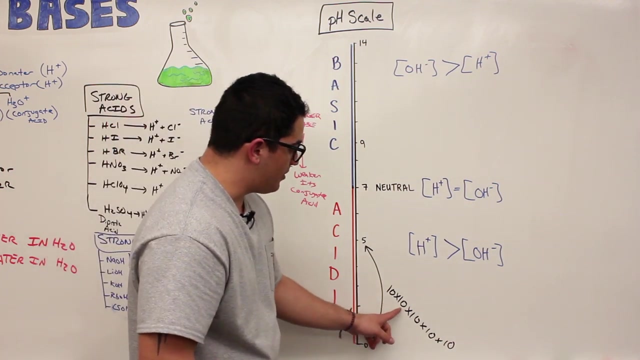 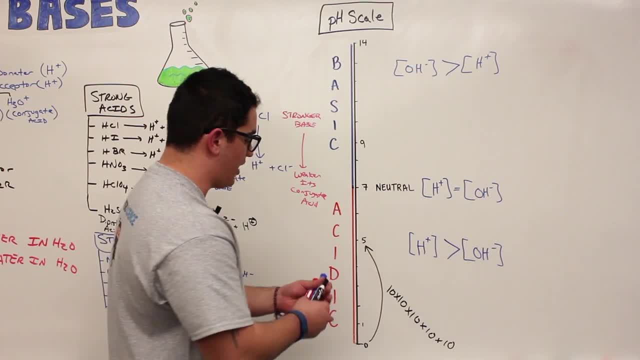 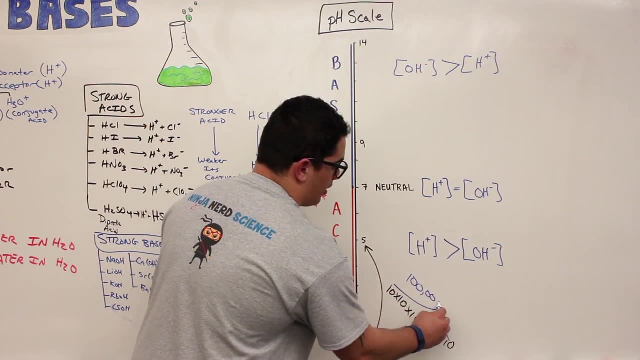 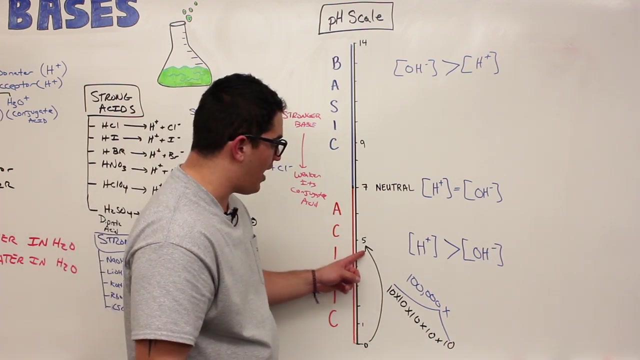 going to be a hundred thousand fold change. That is a hundred thousand fold change. So how much of a change was it? It was a hundred thousand times change. So remember that Whenever we're saying: okay, what's the pH change going from 0 to 5?? Well, each change is a tenfold increase. 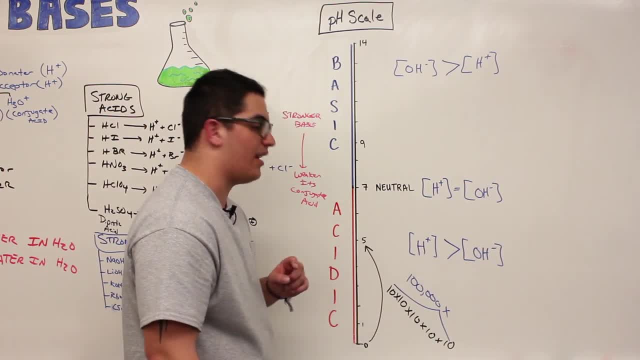 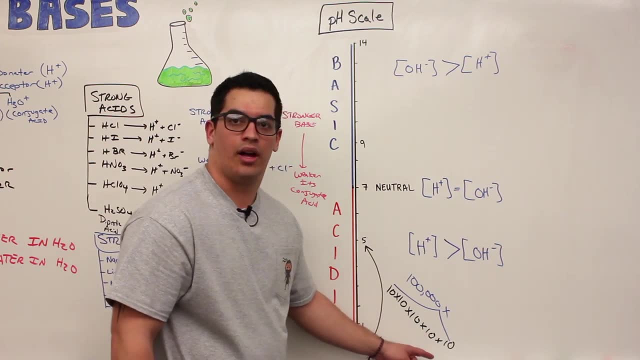 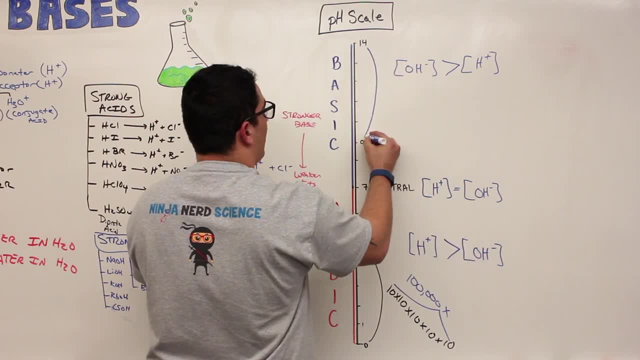 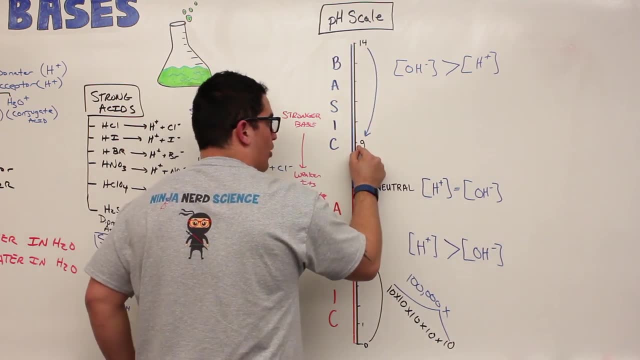 if I'm going all the way from 14 to 9, what am I doing? It's changing by a tenfold scale. So 10 times 10 times 10 times 10, and then over here to this guy, times 10.. So same situation. how many was that? We went from 14 all the way to 9. 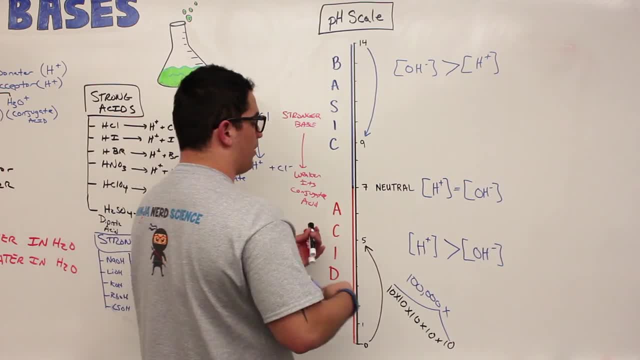 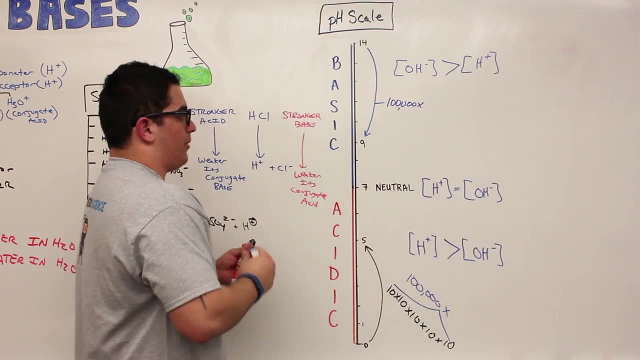 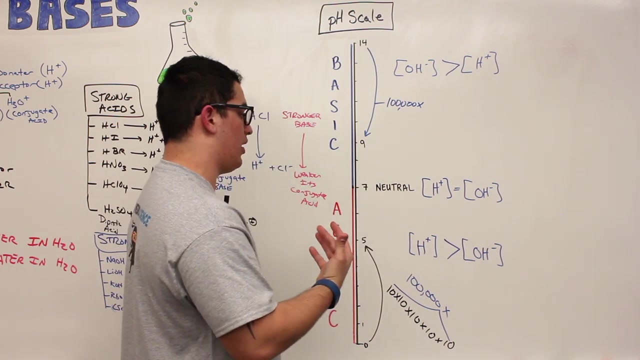 most people be like: oh, that's a five times difference. No, it's a hundred thousand times difference, because it's a 10 times each one. Okay, now another thing: when- because it's this, this base- calculate our number, the sum of all of the numbers, there is a 10, if you will. 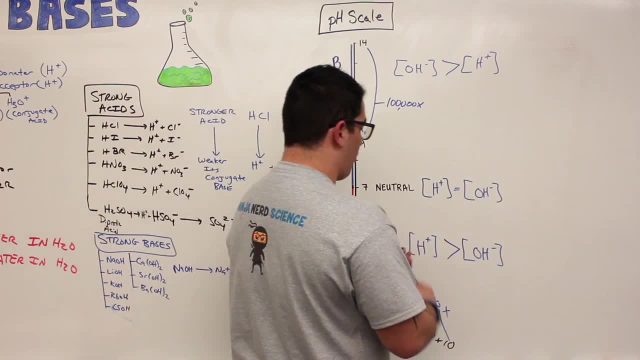 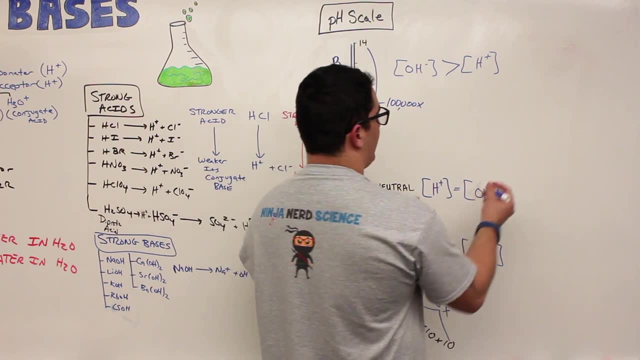 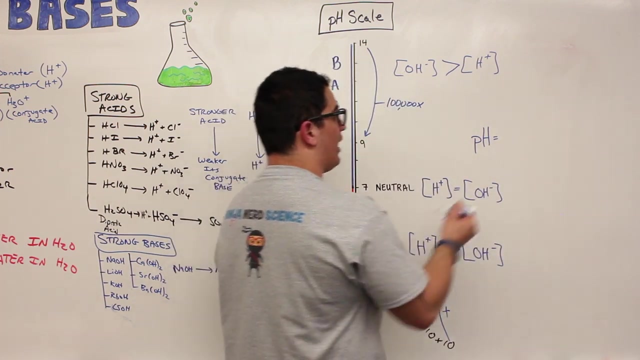 change. They came up with a way to be able to calculate a specific number, which we call this, this pH. right, and so what they said is: okay, well, we can technically figure out what the pH of a solution is, since we have this scale now. and what they said is: we can actually say that pH is equal to we put a negative. 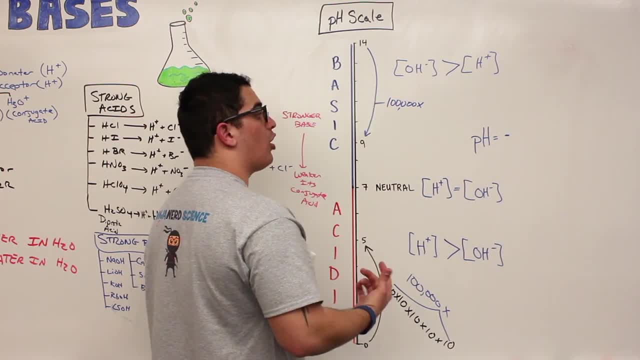 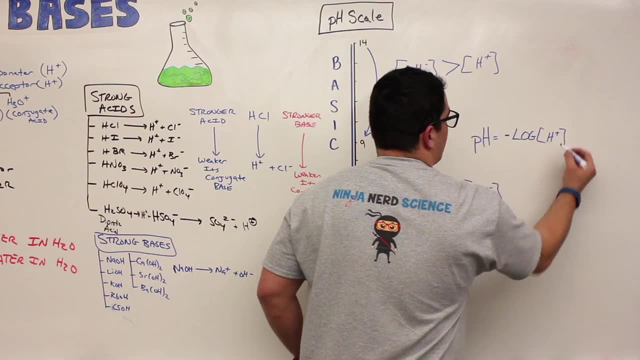 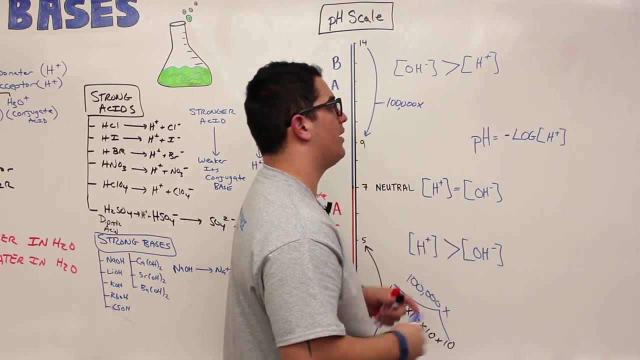 in there for specifically mathematical sake and scale. So pH is equal to the negative log of the H plus concentration. Okay, and that's how we derive this formula to solve for pH. We said it's based on this logarithmic scale, which is a base 10, right, 10-fold change. Same thing, that's. 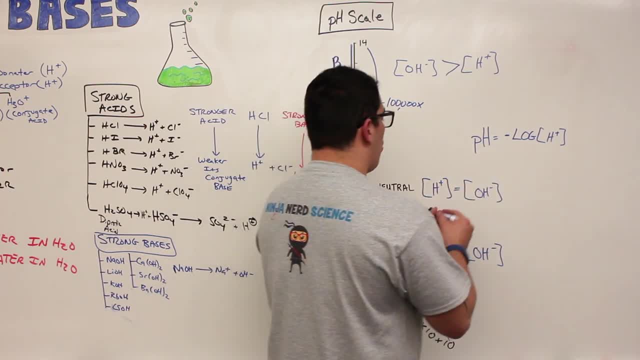 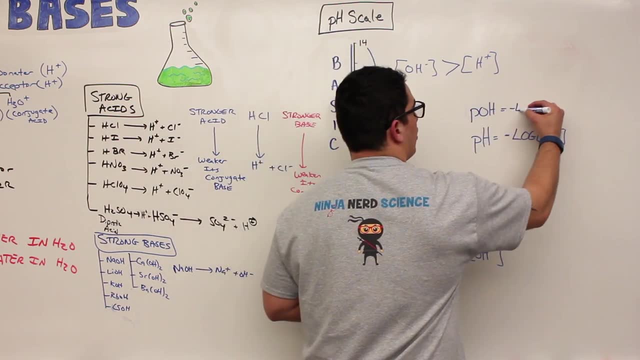 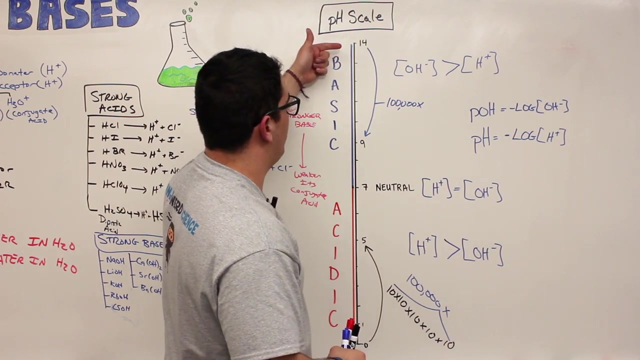 pH. So that would give you the H plus concentration. pOH would give you the hydroxide ion concentration, So it's the negative log of the hydroxide ion concentration. Okay, well, that's cool, because now I have this ability to. 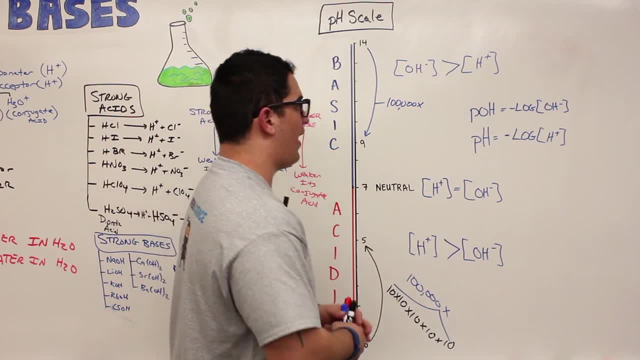 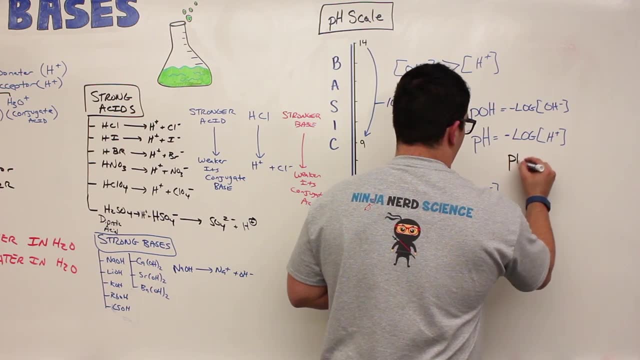 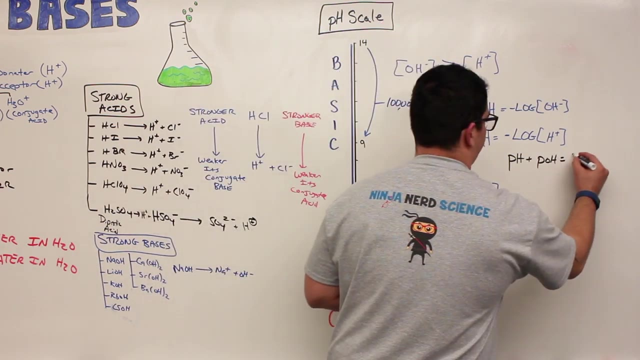 calculate pOH. I have the ability to calculate pH. What if I add both of these two together? So then I take and I add pOH plus pH. That gives me a specific formula: pH plus pOH. Wait, isn't that the whole scale? It is, So it equals 14.. And 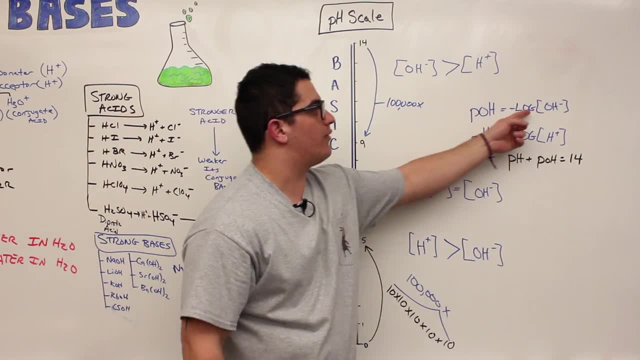 that's how we got along, All right. so we're going to solve for 14.. Let's give it a try. So we have a lot of these formulas, right? So what do we have so far? We have: pOH equals negative log of. 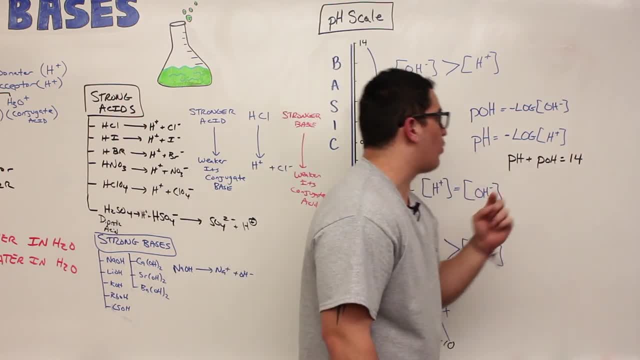 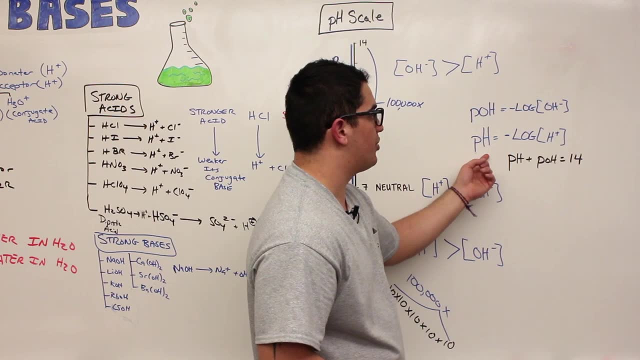 the hydroxide ion, pH equals negative log of the hydronium ion, and then pH plus pOH equals 14.. In the same way, if you know your algebra, if I wanted to solve for hydrogen ion concentration and they gave me the pH, well, knowing my 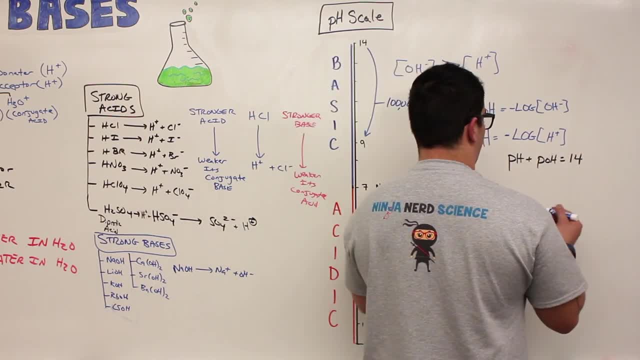 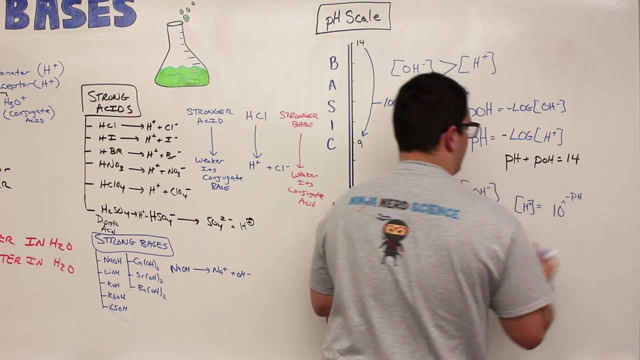 logarithmic relationship. it's a base 10.. So it's going to be 10 to the negative pH. So if I wanted to solve for hydrogen ion concentration, that formula would be H, 10 to the negative pH. If I wanted to solve for hydroxide ion concentration, all I would 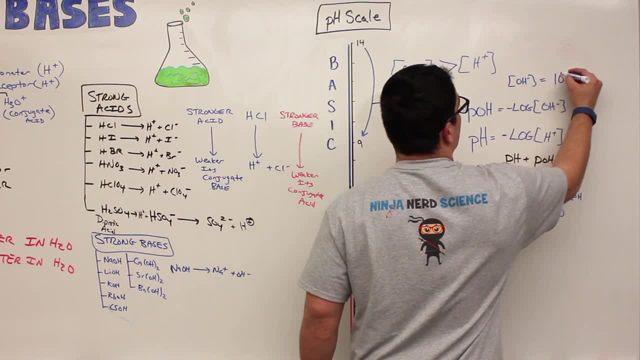 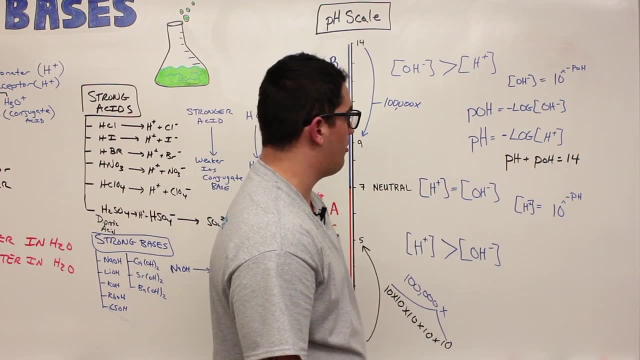 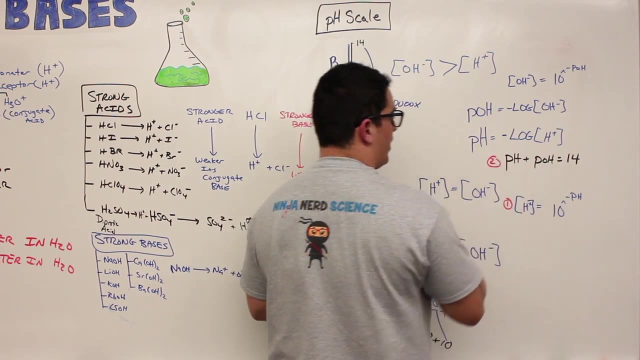 do is I'd take 10 to the negative pOH So I can move all the way around this pH scale right. So again, how many formulas have we been able to come up with here? We came up with: H plus equals 10 to the negative pH. pH plus pOH equals 14, pH equals negative. 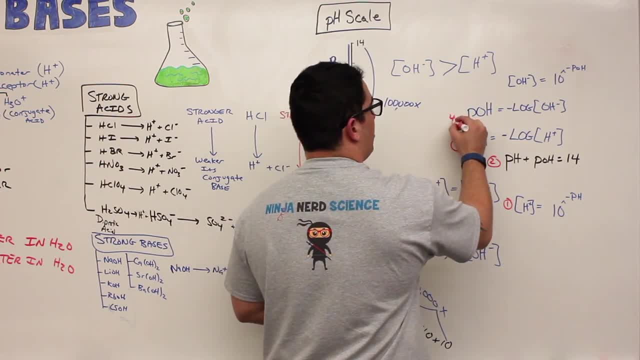 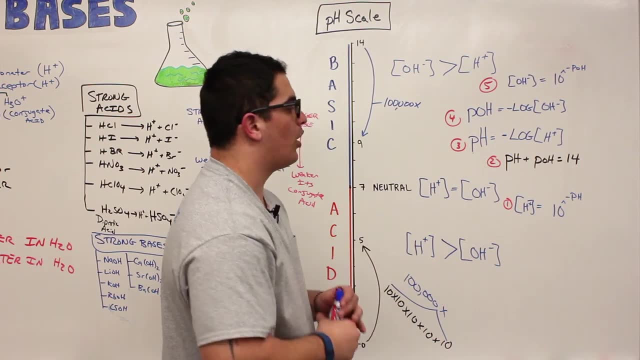 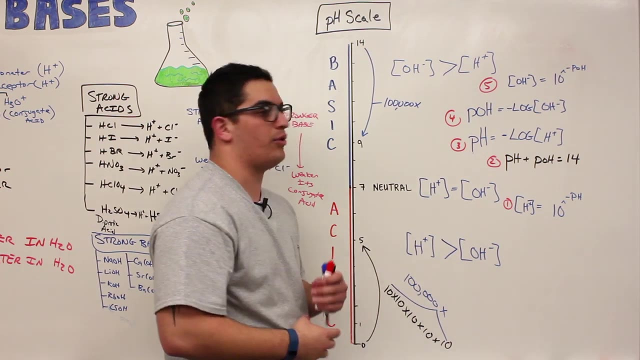 log of the hydronium ion. pOH equals negative log of the hydroxide ion, and hydroxide is equal to the 10 to the negative pOH. One more thing I want to talk about here. Okay, water has the ability to act as what's called amphoteric, meaning it can act like an acid and a base. 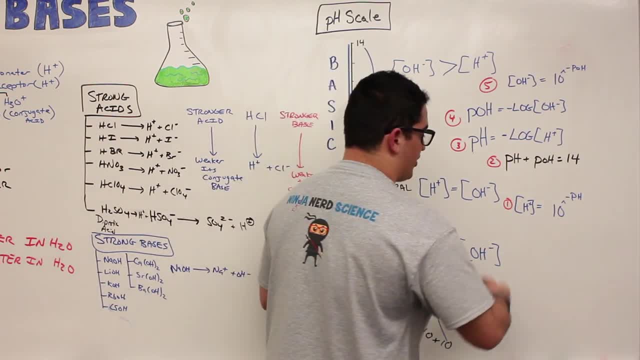 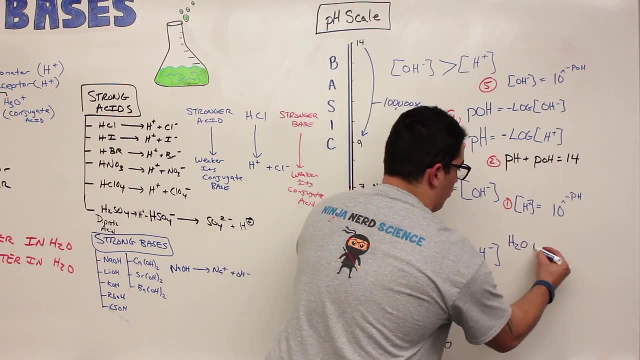 And there's other molecules that can do that. So when water actually disassociates, right, So say, here's water, Water disassociates, Let's say it reacts with two, two waters react And when it- or we can say it- autoionizes. 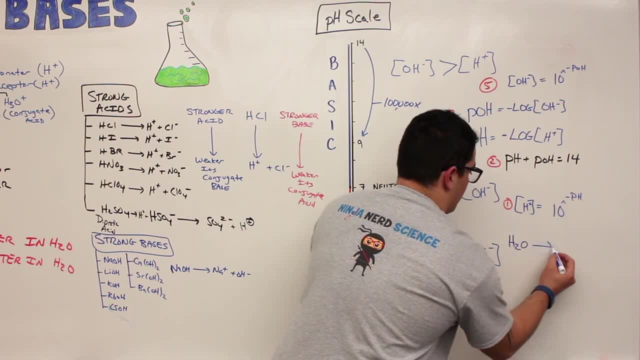 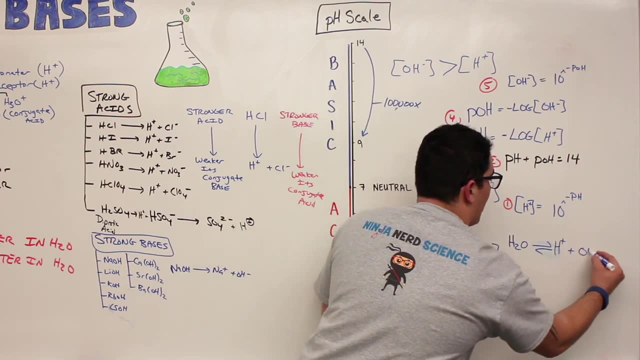 When it autoionizes. let's actually just do that, Say it's autoionizing- right? When it autoionizes, it produces an H plus and a hydroxide ion. Okay, that's cool, right, Because I just 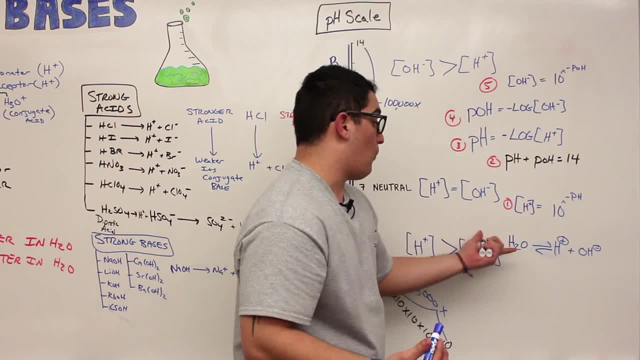 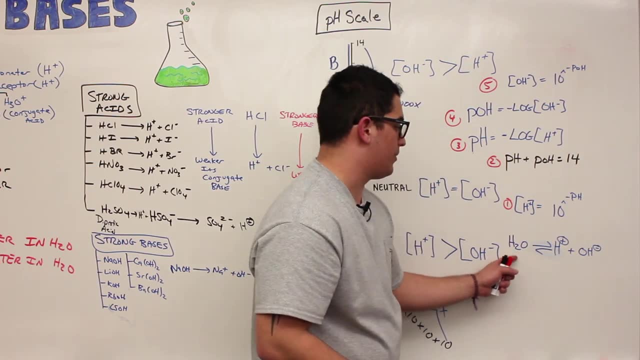 kind of like I know what H plus is and I know what hydroxide is And I know what water is. Well, we actually were able to calculate a rate at which this actually occurs. So, with the rate at which water autoionizes, and we said it's defined as Kw And Kw is equal, 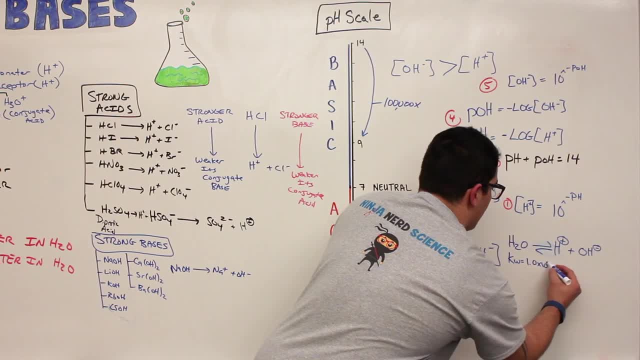 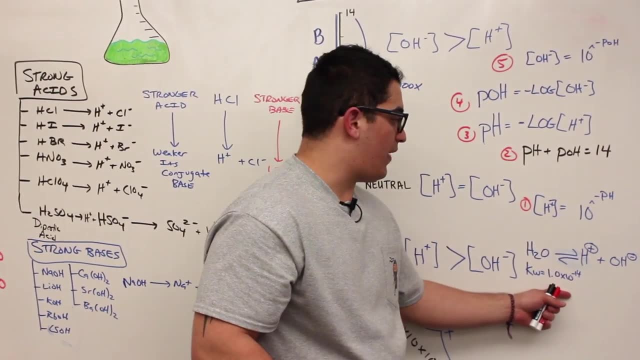 to 1 times 10 to the negative 14.. So that's that rate. That's the rate and that takes a long time. So that's a very. you know, it's a very, very small, small number, right. 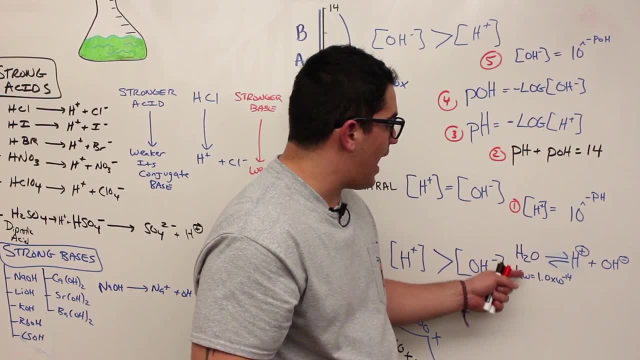 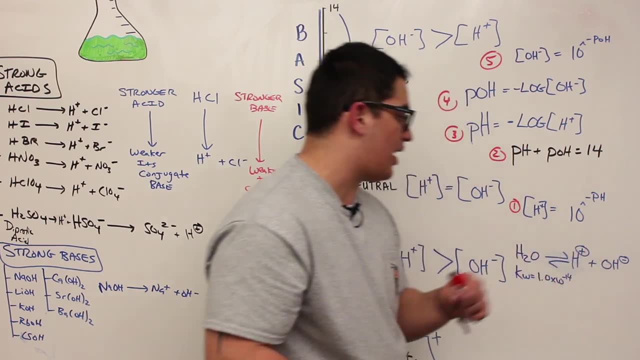 So very, very, very small number. So with this, what's happening is the autoionization of water. you have a specific rate at which this reaction occurs to produce H plus and hydroxide ions. So we can actually say one more thing. Okay, well, I know that Kw cause. 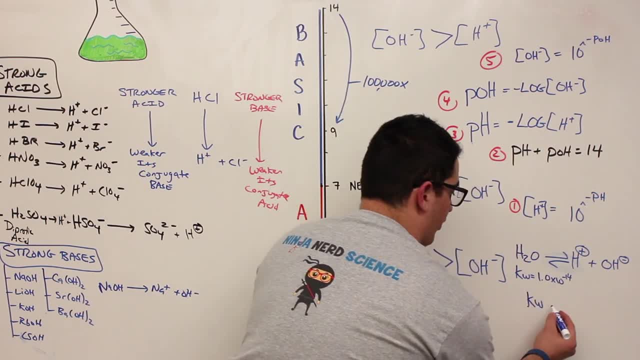 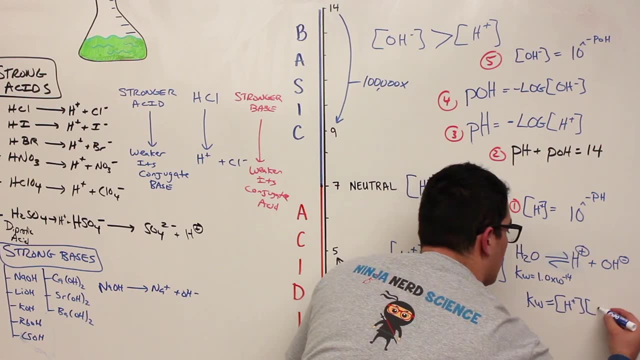 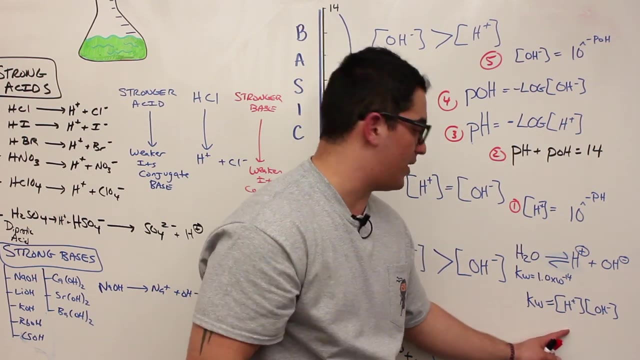 I'm producing these guys is equal to the H plus concentration times, the hydroxide ion concentration. So at any point in time here I could rearrange this formula. I can get three other formulas from this. I could have this formula and I could have H plus equals. 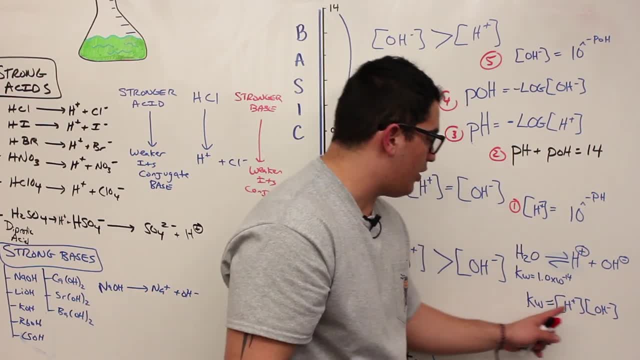 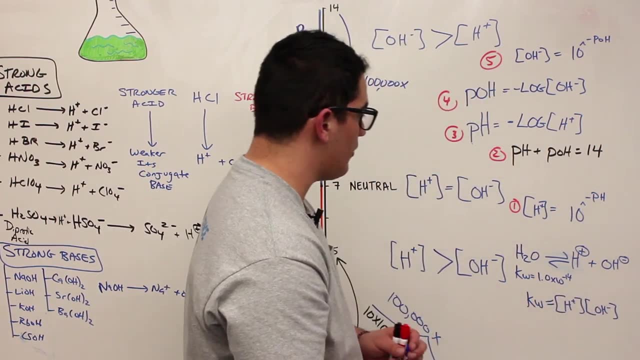 KW over hydroxide, or I could have: hydroxide equals KW over H plus. So there's a lot of different formulas I could derive from that, But this gives me the relationship of KW. All right. Now let's talk about one other thing here, And that's going to be talking about weak 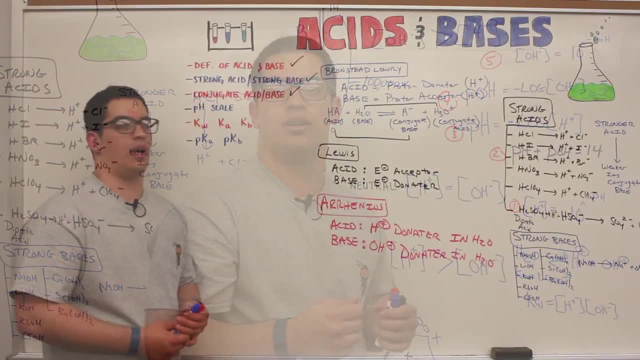 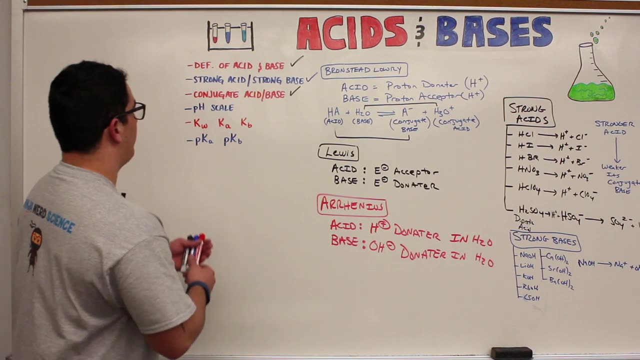 gases and weak bases very briefly, And then we're going to go into a lot of calculations. All right, So we finished up talking about the pH scale. We talked about POH, pH H plus hydroxide KW. So what have we finished so far? We've talked about the pH scale. Okay, Again. 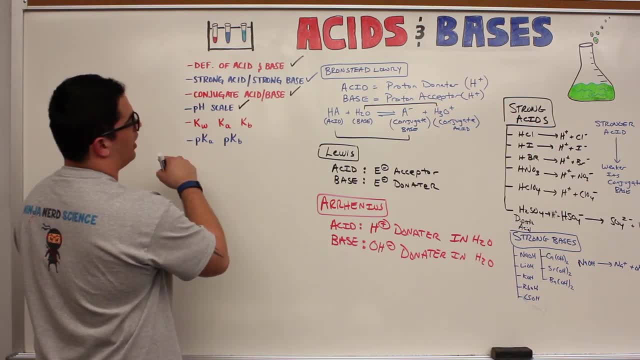 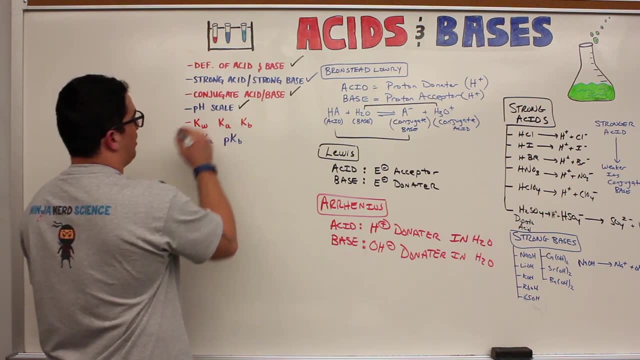 we talked about the logarithmic scale, H plus hydroxide. We talked about acidity, basicity. We talked about KW- right, So we talked about KW. Now we got to talk about KA and KB, PK and PKB. 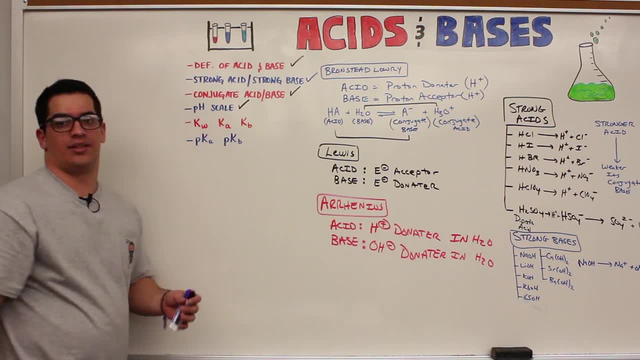 So right now, we've only been talking about strong acids and strong bases. So we have to get just a baseline definition of what's well, what's up with these weak acids and weak bases. So I'm going to go ahead and talk about the pH scale. So I'm going to go ahead and talk about 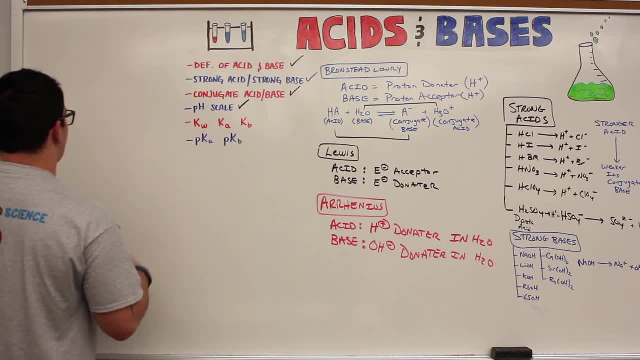 the pH scale. So I'm going to go ahead and talk about the pH scale. So I'm going to go ahead and talk about going to give you an example. first off, let's just do a weak acid. So an example of a weak acid could be: I could pick acetic acid, So I'm going to pick acetic. 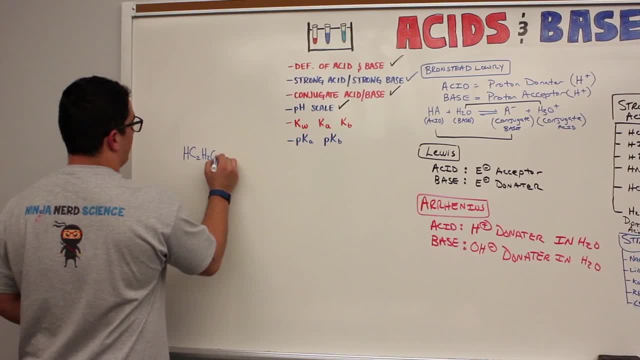 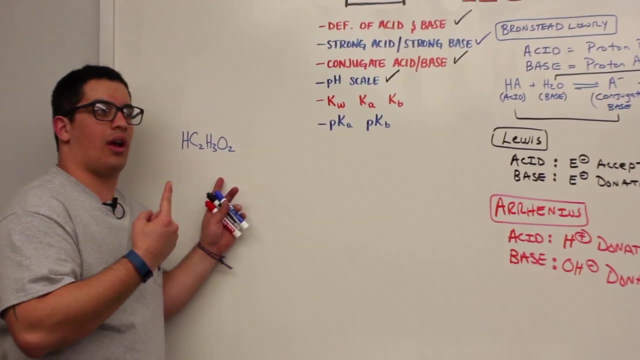 acid, I'm going to say HC2H3O2.. Acetic acid is a weak acid. Why is it a weak acid? What was a strong acid? That means that the strong acids are defined as completely disassociating, giving all of their protons up. So if I have put in a 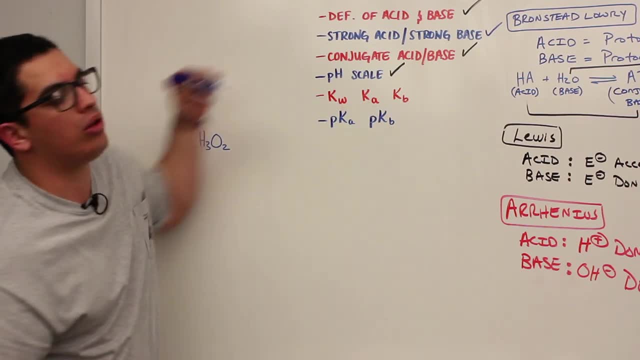 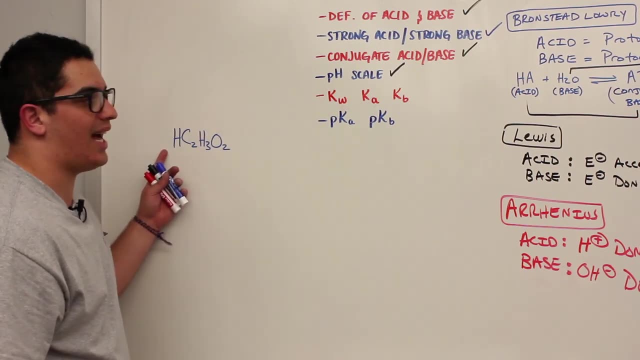 0.1 molar solution of hydrochloric acid, all of that 0.1 molar will go over to forming H plus and Cl. If I put a 0.1 molar solution of acetic acid into solution, not all of it, not all that 0.1 molar will get converted over into H plus. 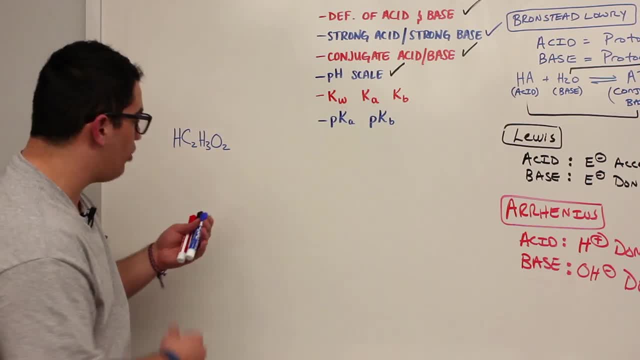 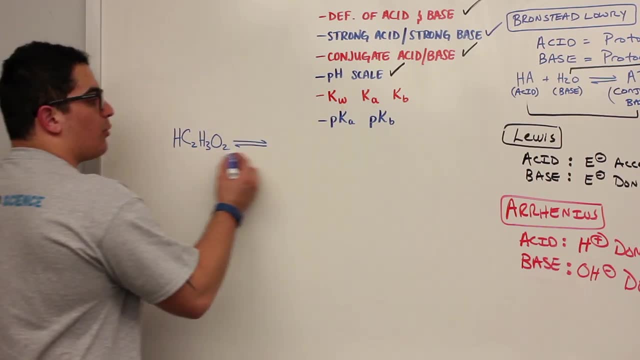 and acetate. Why? Because not all of it disassociates. So now what we say is: let's say that we take this reaction. it's a double arid reaction. So in other words, this can occur. it can actually be an equilibrium. So whenever he gives up, 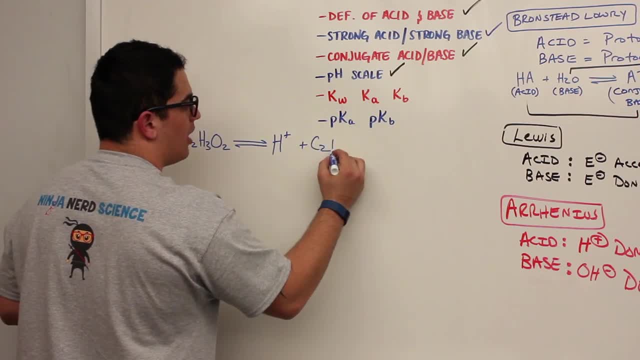 his H plus, he'll give up his H plus and he gives up and he flies it. I'm going to say that I'm going to fly it, but I'm going to forms these two structures. and again, what would this be? Weak acid? this would be its. 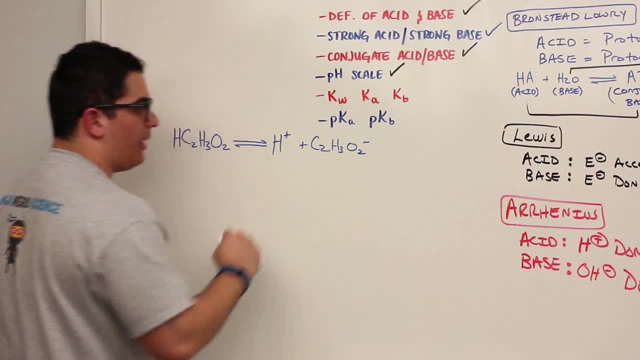 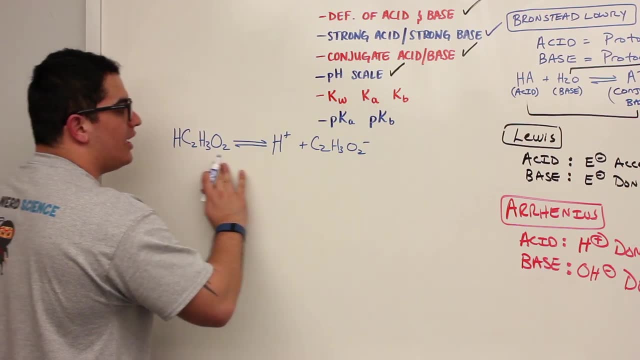 conjugate base. So that's the weak acid conjugate base pair. and if I did this in water, water would be the base and H plus would be the conjugate acid. All right, so now, because he didn't disassociate completely, we have to have some type of number, or rate if you will, to determine how. 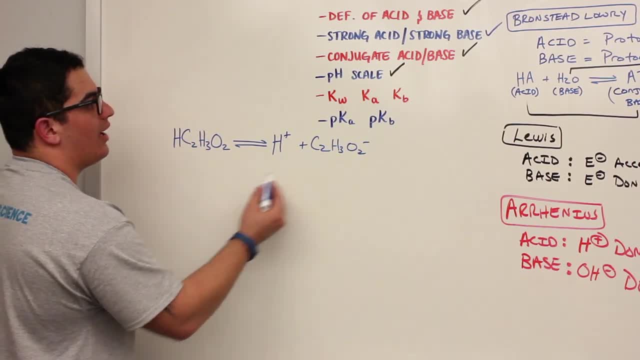 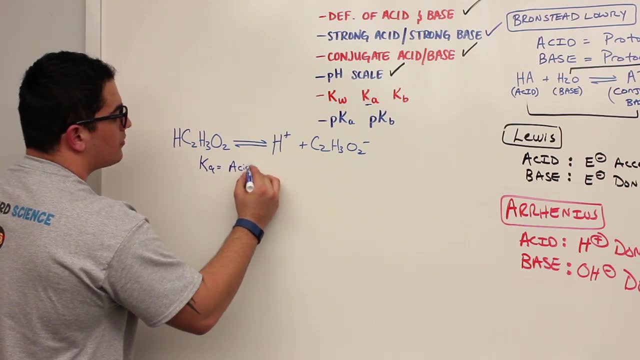 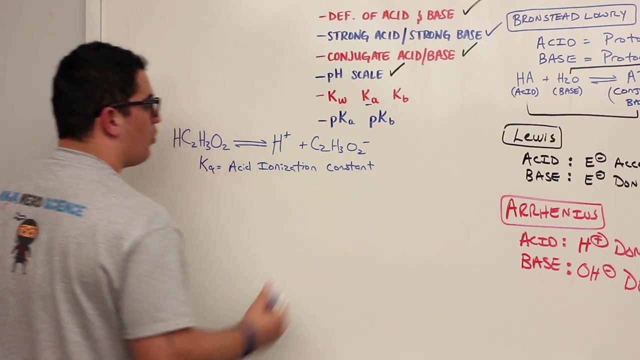 much of that H plus disassociates. So what do we use for that? That's where Ka comes into play. Okay, so Ka is defined as the acid ionization constant. In other words, it gives us how much of this acetic acid disassociates into a solution. Okay, how much of it goes into H plus. Now 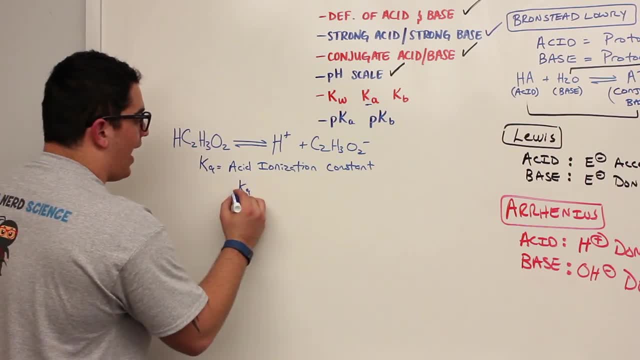 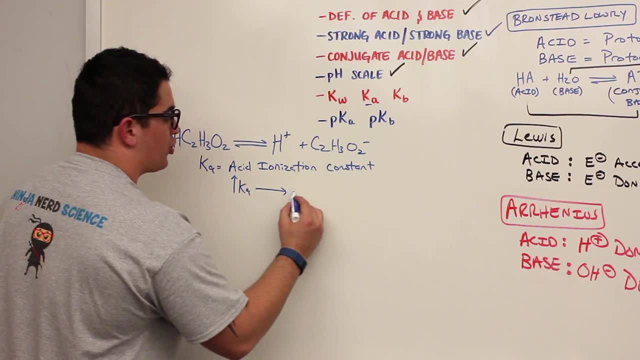 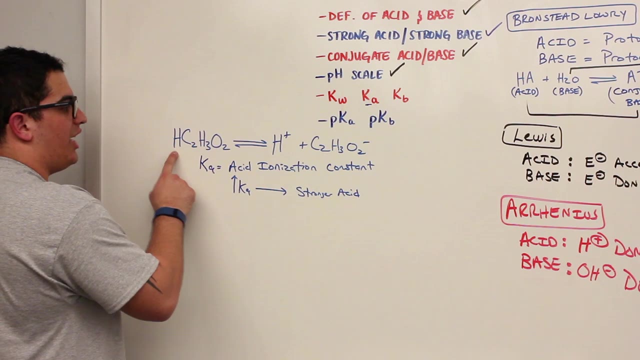 here's what we need to know out of this: The greater the Ka, all right. so the more that Ka, the larger it is. The larger the Ka, the stronger the A. Okay, in other words, the bigger this is, the more H pluses are going to disassociate, Okay. so if I were to do, 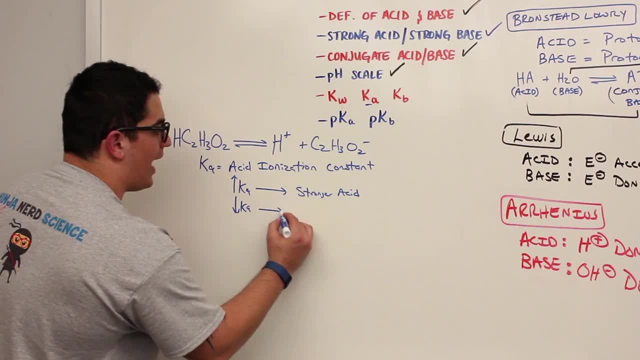 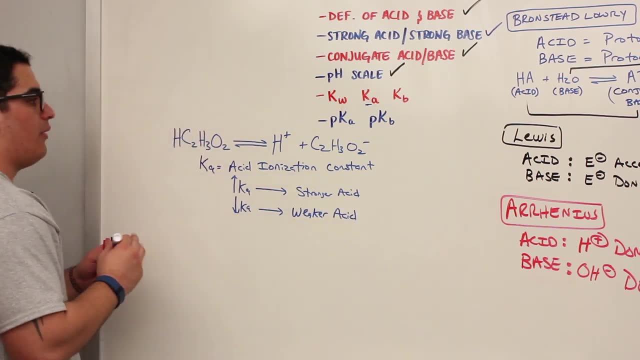 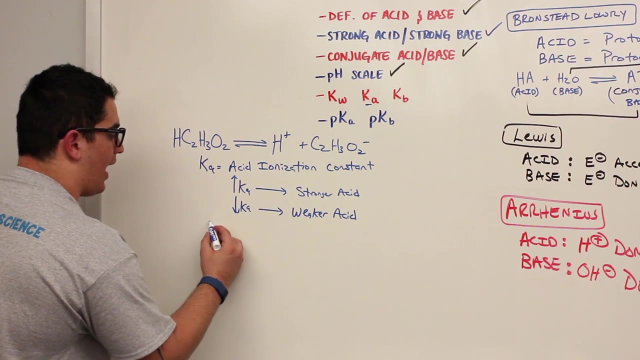 something like this: a low Ka. a low Ka implies a weaker acid. Okay, cool, While I'm here, let's just talk about P Ka. So P Ka, you can actually calculate it, because P Ka is the acid ionization. 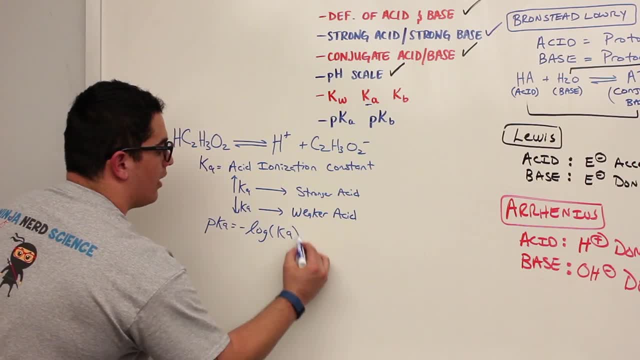 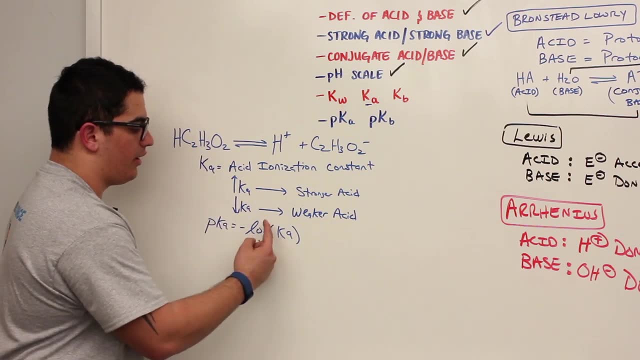 constant. P Ka is the negative log of the Ka. Okay, so now, if I said that a Ka, if it was really, really big, and I wanted to try to be able to figure out P Ka, P Ka is the actual opposite. So now we 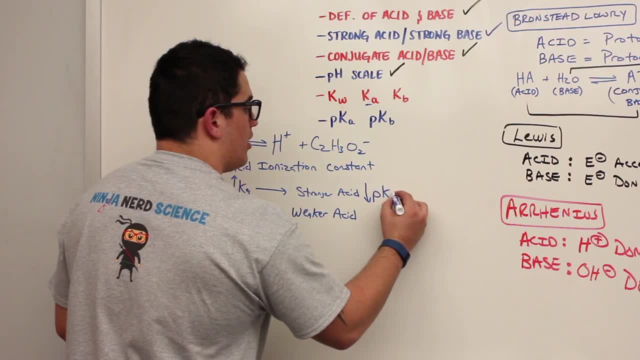 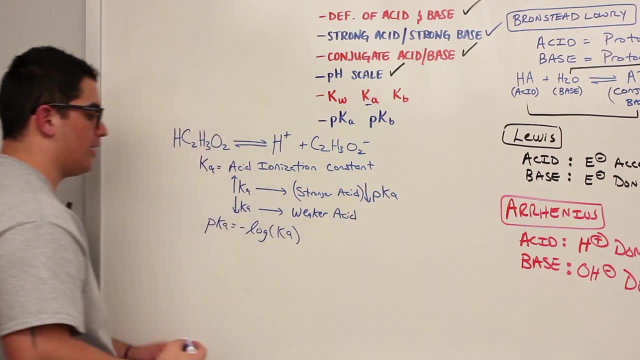 say: the lower the P Ka, the stronger the acid, The higher the Ka. the lower the P Ka, the stronger the acid. because it's going to give you this log amount And again we can actually solve for Ka How: 10 to the negative P Ka. So Ka is equal to 10 to the negative P Ka. 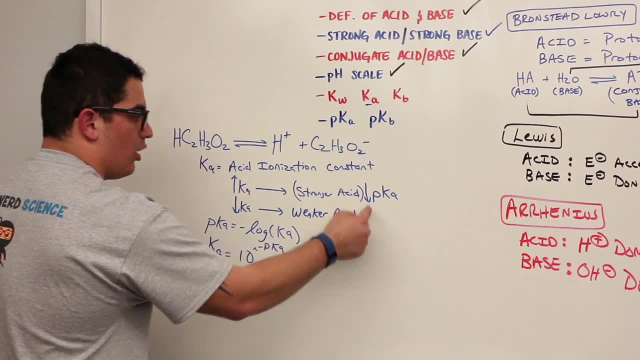 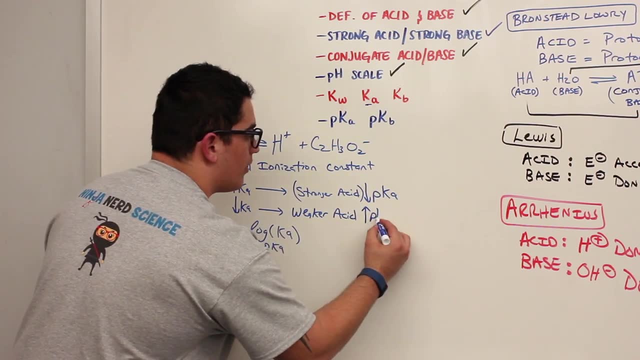 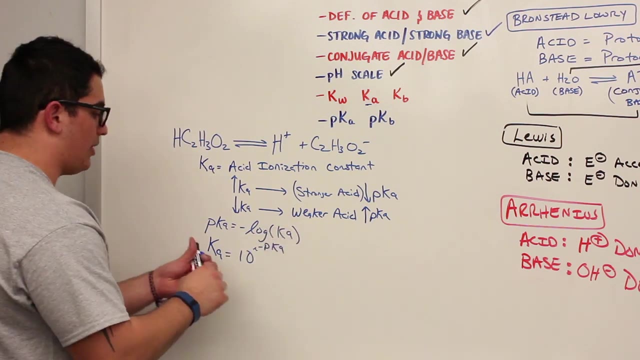 So you can solve for that relationship. So again, higher the Ka, stronger the acid, Lower the P Ka: stronger the acid, Lower the Ka. the weaker the acid. The higher the P Ka, the weaker the acid. Okay, Now and again, weaker acid would imply pH, So you could say this would be a. 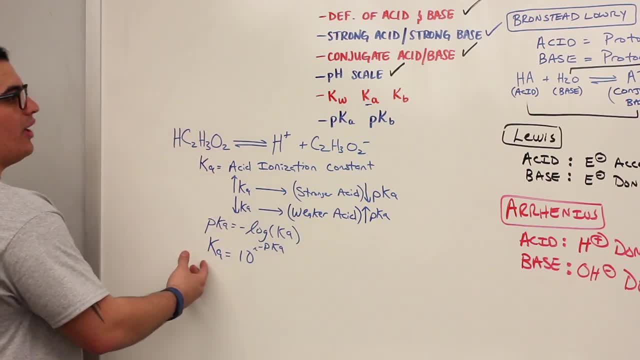 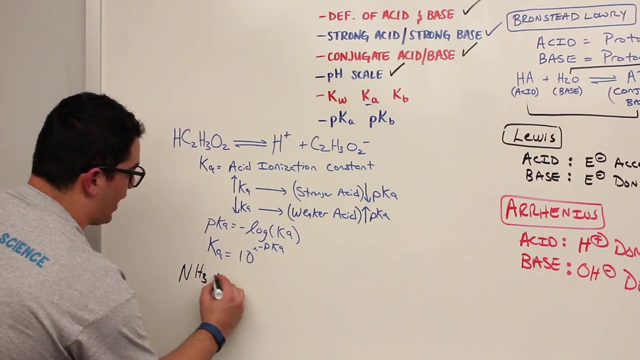 low pH. this would be a higher pH. Now let's go ahead and talk about weak bases. So if I talk about weak bases here, let's say I use ammonia, So I use ammonia, So NH3. And I take NH3 and I react him with water. 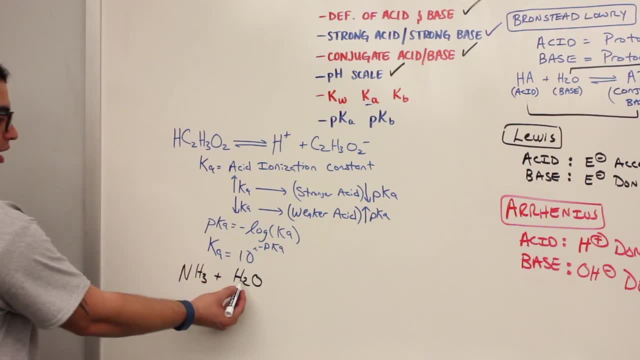 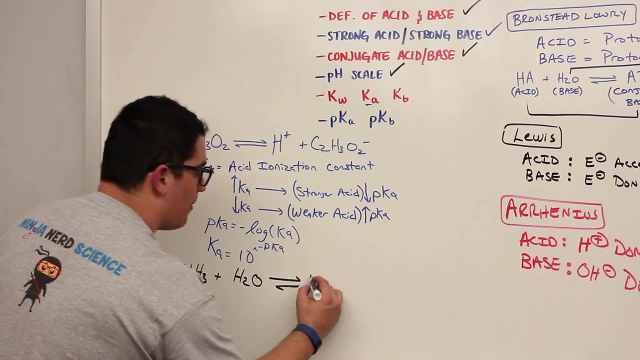 What's the definition of a base? A base accepts protons, So in this case he has to accept a proton. From who Water? So water gives up a proton, puts it on to ammonia and converts him into ammonium, which is a weak acid. So there's our base conjugate. 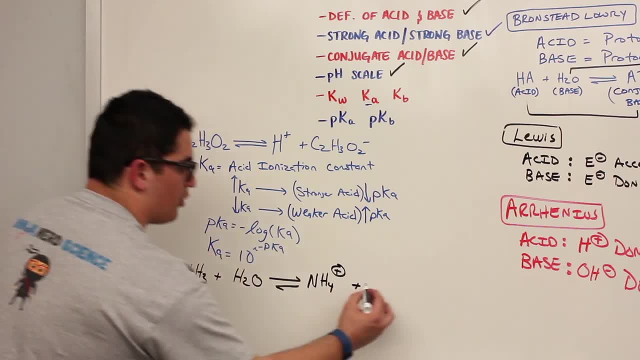 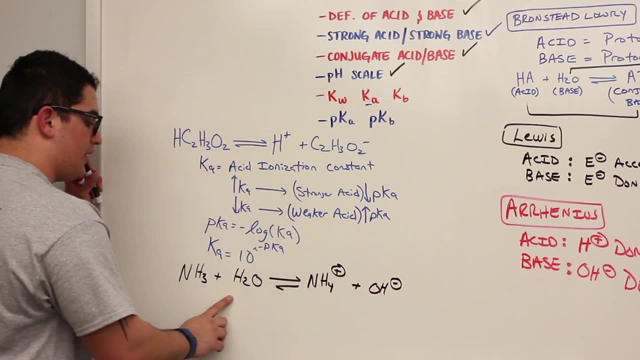 acid pair, And then H2O gives up a hydrogen, So it turns into hydroxide. So there is your acid conjugate base pair. Now, same thing. Ammonia is not a strong base, So it doesn't accept protons as readily. 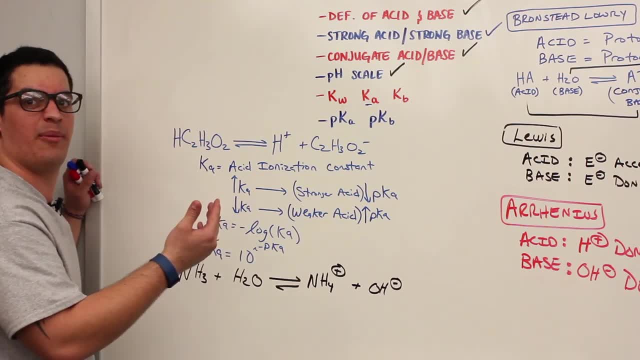 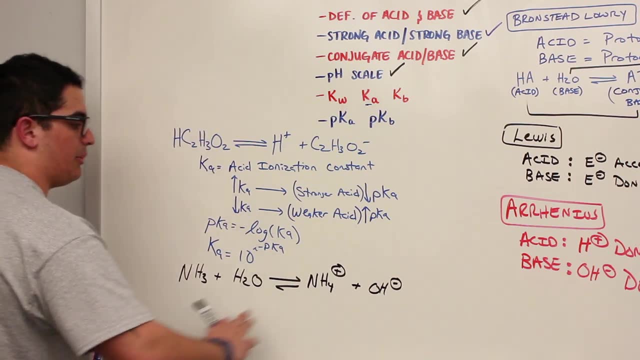 And it doesn't produce hydroxides as readily as something like sodium hydroxide. So we have to get another type of constant, if you will, to determine how much of this hydroxide is being produced, or how much hydrogens is he accepting. 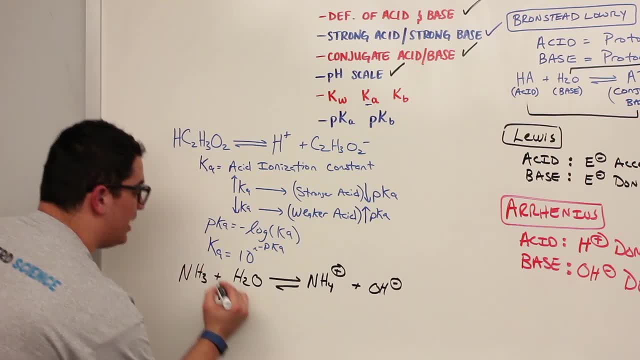 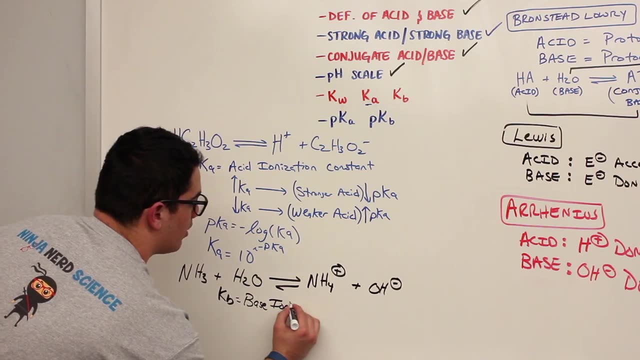 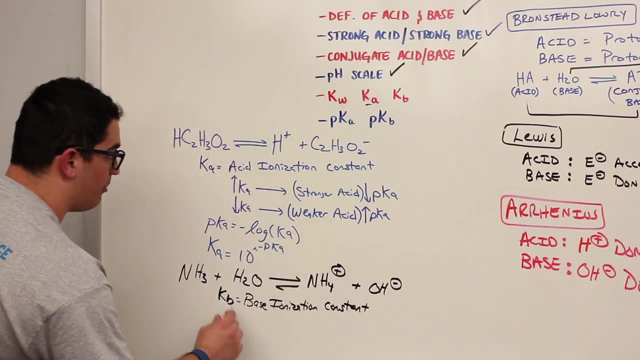 So we give that a Kb, okay. And Kb is the base ionization constant- okay, and it's the same thing we did up here with the Ka. So the higher the Kb, but remember we've got to be careful now- the higher the Kb, the stronger. 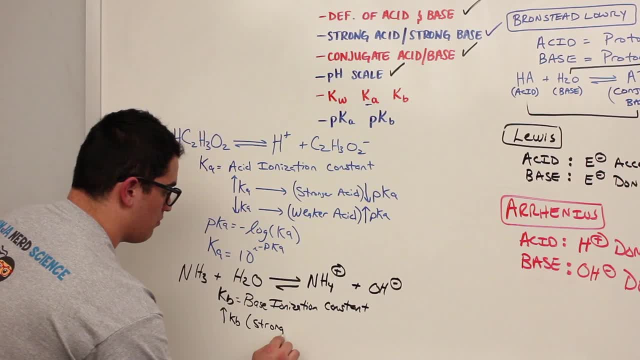 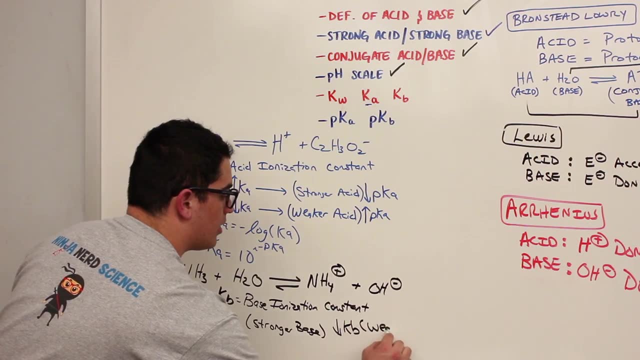 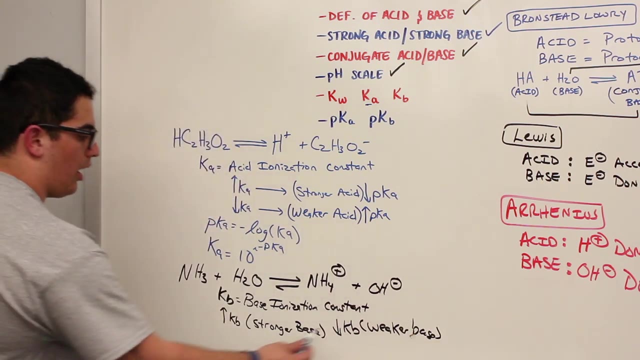 the base okay. Stronger the base, The lower the Kb, the weaker the base, okay. And the same thing is applied with the PKBs. and so PKb here. if I were to say for this one, if it has a high Kb it has to have a low PKb, and if it has a low Kb it has to have. 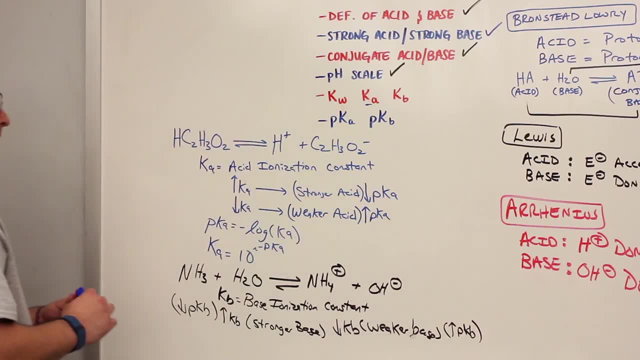 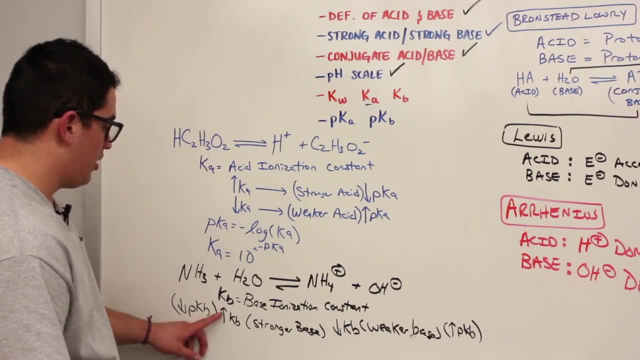 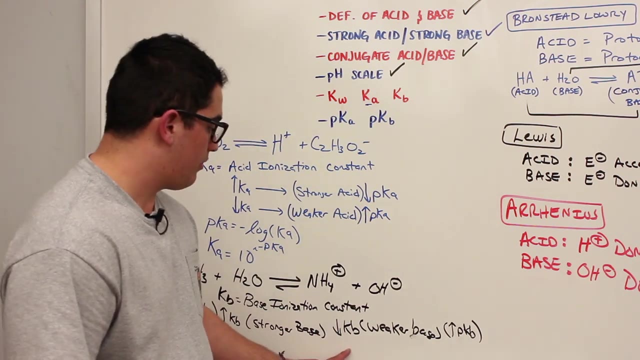 a high PKb, Okay, All righty. So again, these are your inverse relationships here. So the higher the Kb again, the lower the PKb. so that's going to be a stronger base in this condition, And if there's a low Kb it's a weaker base and if it's a weaker base it's going to have. 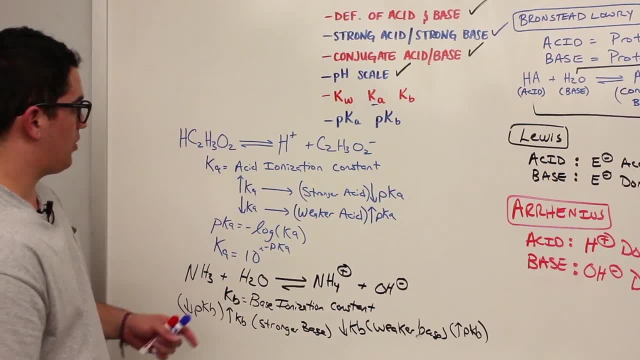 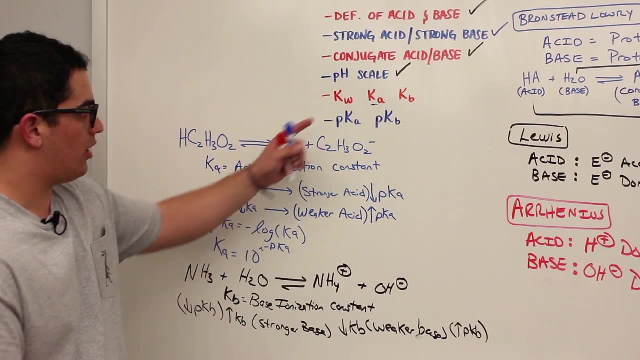 a high PKb, All right. so we finished off talking about Ka and Kb now, right? So let's go ahead and say one other thing here before we go into PKs and PKb's. So I talked about Ka and I talked about Kb, right? 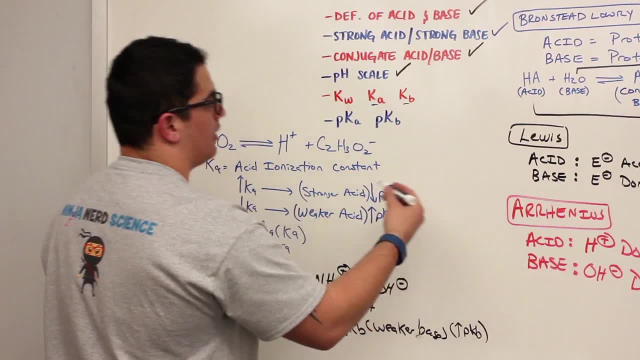 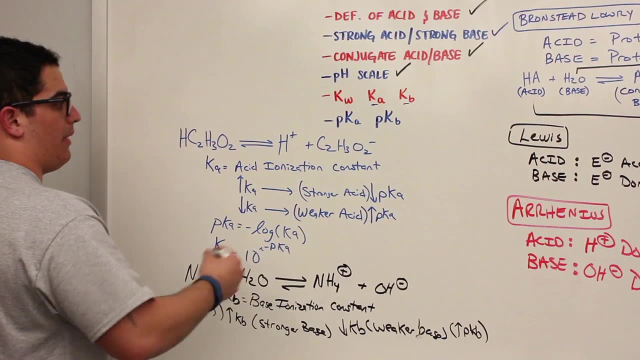 And again, the higher the Ka, the stronger the acid. the higher the Kb, the stronger the base. higher the Ka, the lower the PK. the higher the Kb, the lower the PKb. right And again, that's just a measure of acidity or basicity. 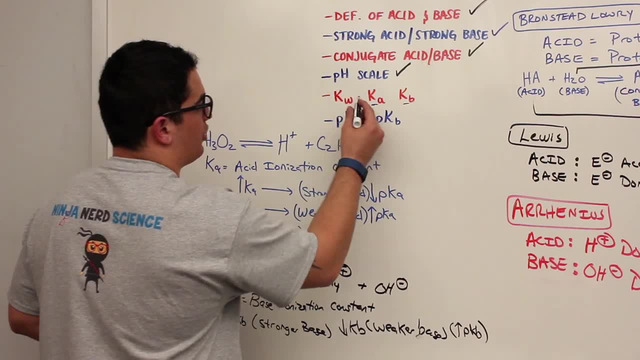 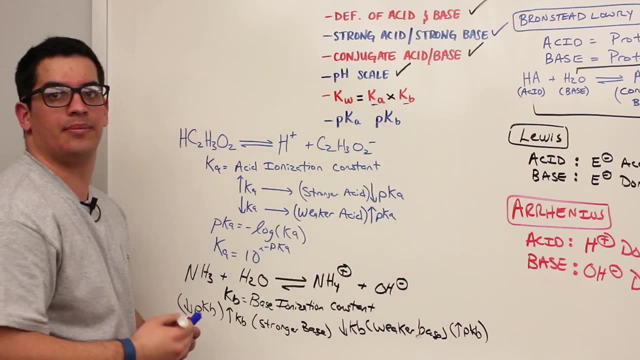 Now what we can do is we can say Kw. this is actually working perfectly. Kw is equal to Ka times Kb. So now, why is that? Why is that? If you remember from before, what did we say Kw was equal to? 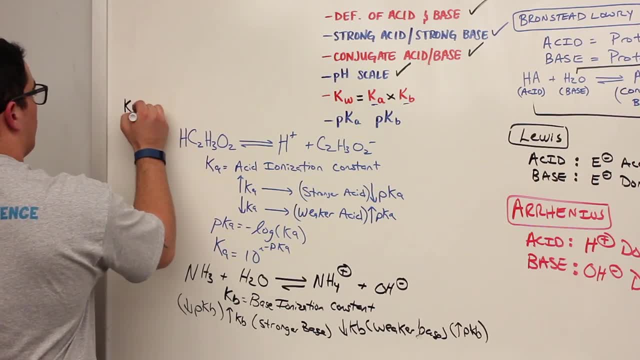 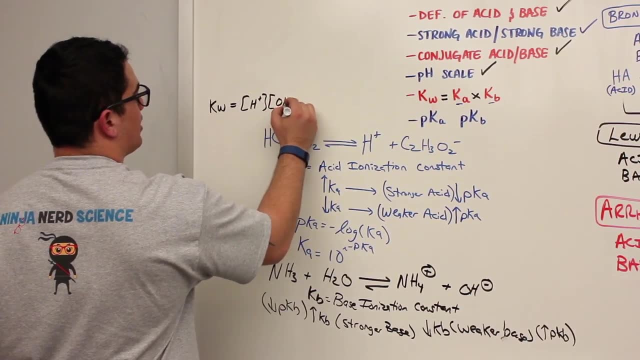 If you remember from before, we said Kw, which was 1.0 times 10 to the minus 14, is equal to the H plus concentration times, the hydroxide ion concentration. right, We talked only about that for strong acids and strong bases. 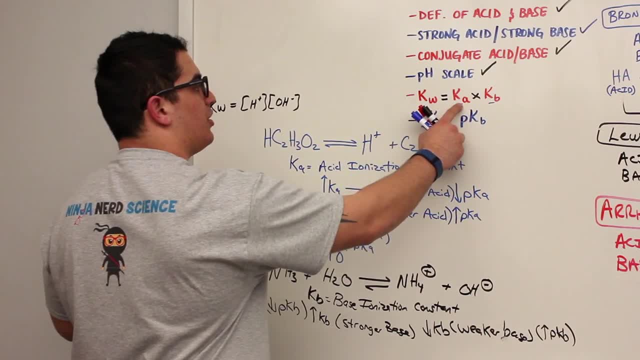 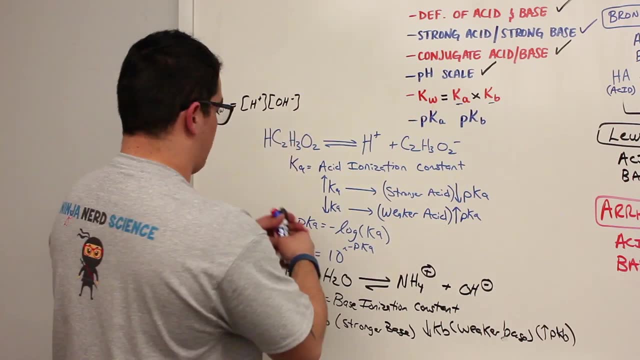 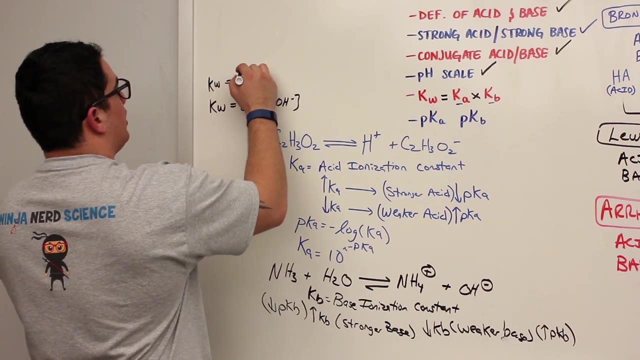 The formula still applies here, but now we just have to take into consideration the amount of the acid that ionizes, and then Kb, the amount that the base ionizes. So then for this case we can actually say H plus We could apply here the Ka, so Kw equals Ka, and then hydroxide. 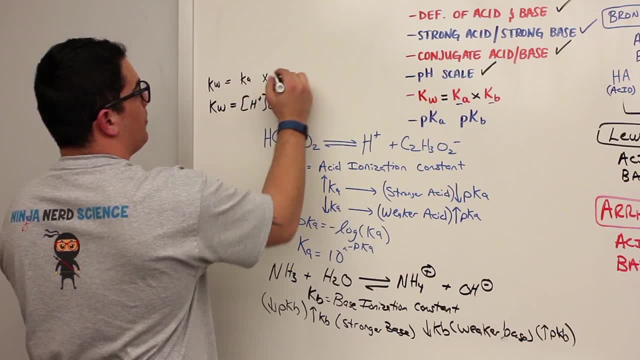 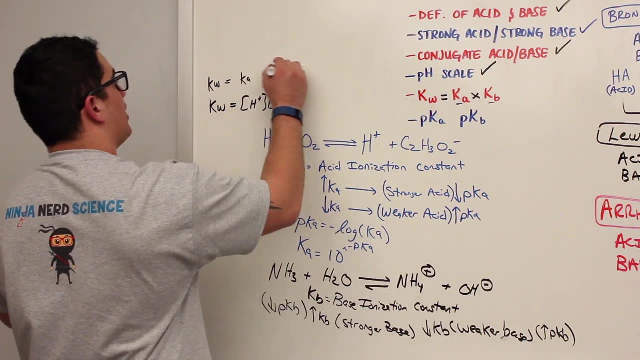 We can say how much of the hydroxide disassociates times Kb, And so we could use this formula once again to be able to determine some of these calculations that we're going to do. okay, So again, Kw equals K times. Kb is an important one. 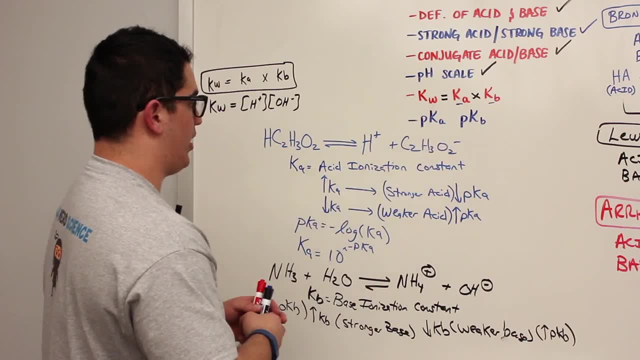 Now let's finish up with PK and PKb. We already know the relationship right That PK is equal to the negative log of the Ka, So we're going to use this formula once again to be able to determine some of these calculations that we're going to do. 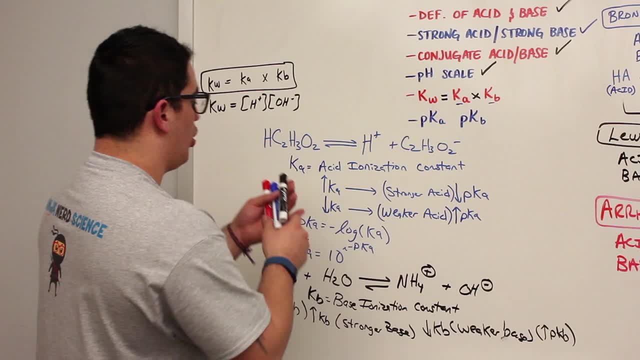 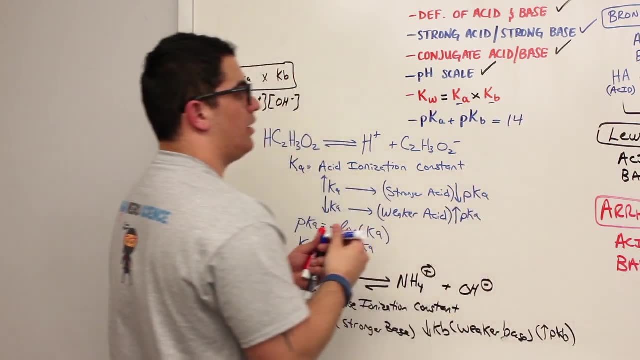 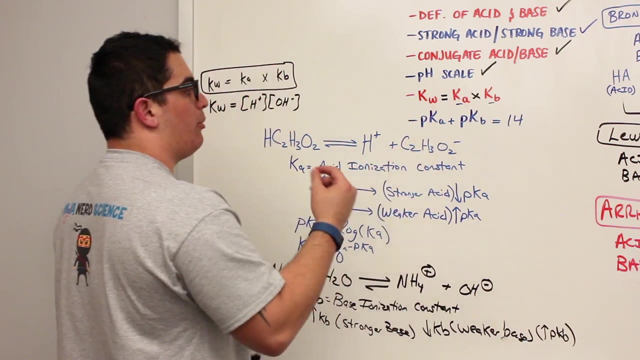 And PKb is equal to the negative log of the Kb. We can actually say Pka plus Pkb equals 14.. Doesn't that sound familiar? Like Ph plus Poh equals 14? Same concept here. Because here's one thing I want to finish up with with Pka and Pkb's. 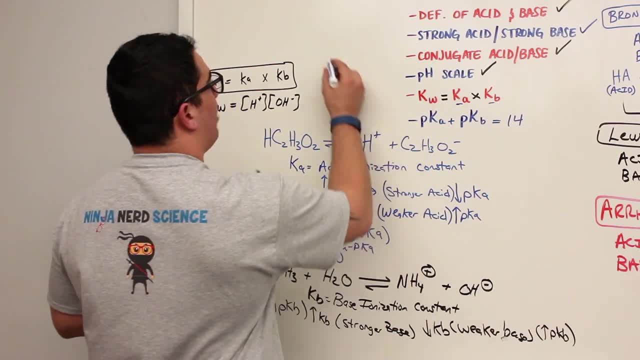 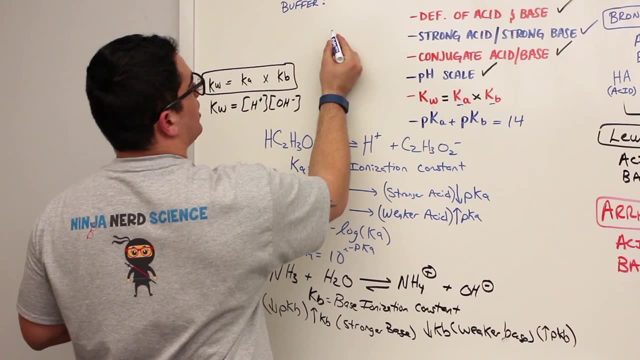 We're going to talk about buffers in our final videos, And a buffer is basically a mixture. So a buffer is designed to resist any abrupt changes in the pH. So a buffer is made up of an acid, a weaker acid. so a weak acid and its associated. 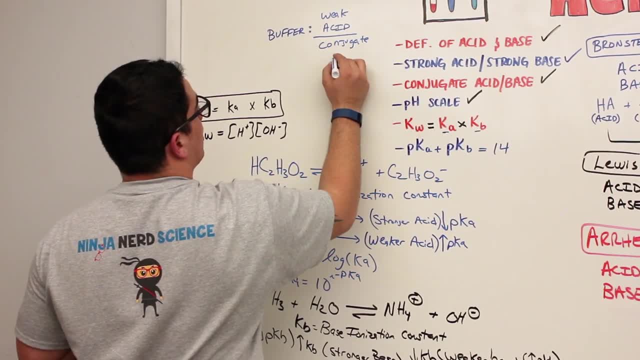 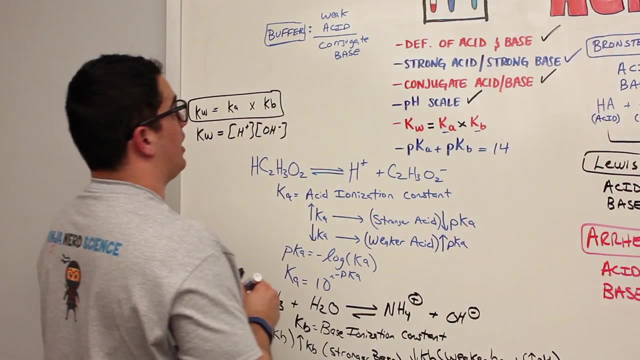 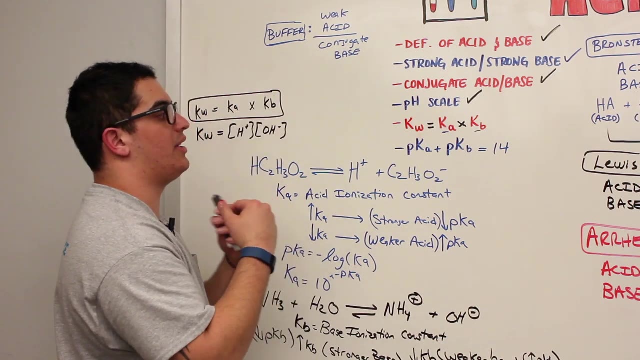 conjugate base. That's what a buffer is. So when we're picking a buffer for maybe some type of reaction in the chemistry lab or within the actual human body, we want to make sure that the buffer that we're applying is pretty darn equal to the pH that we desire. 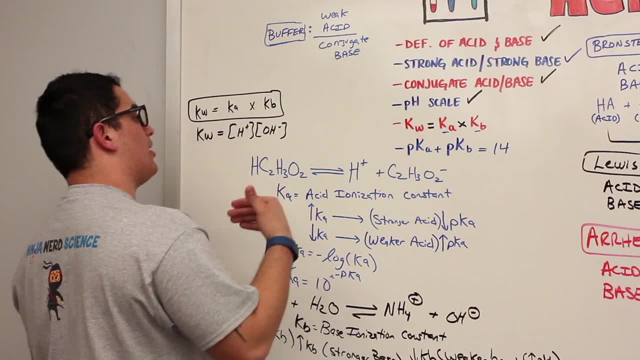 So, for example, my blood is naturally going to keep a pH of about 7.35.. So I'm going to go ahead and do that. I'm going to go ahead and do that: 7.35 to 7.45.. 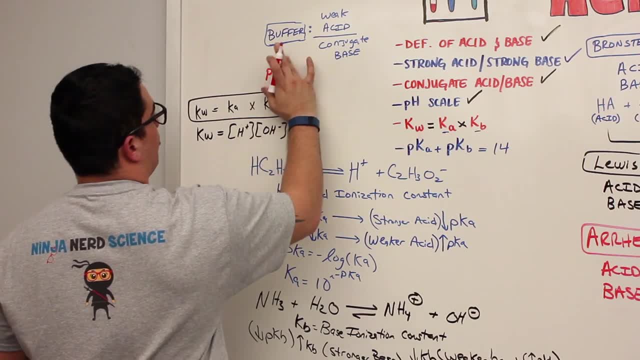 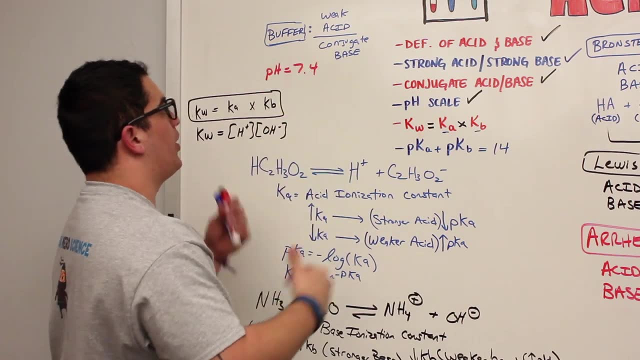 So let's say that's the pH. Let's just say 7.4 to keep it right in the middle, right, Keep it a nice number here, 7.4.. If I had to pick between a whole bunch of different buffer systems that I'd want in. 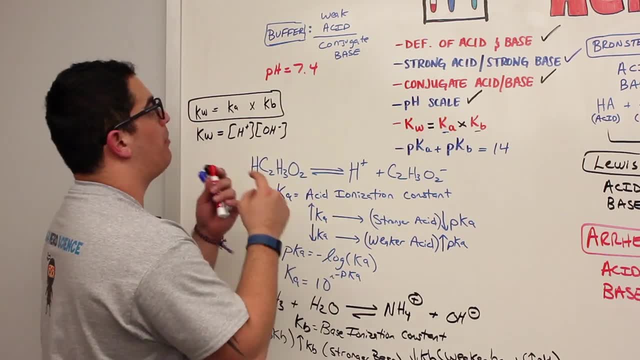 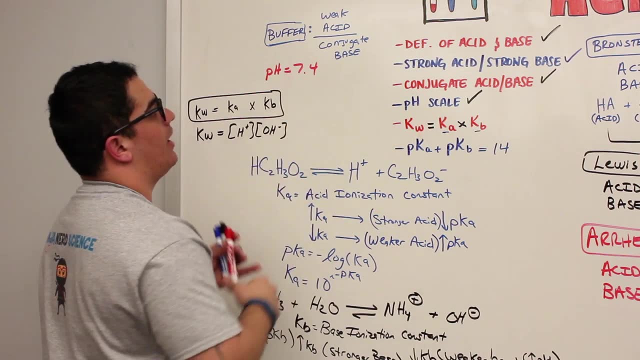 my bloodstream to keep it at that part right there. I'd want the Pka of a buffer to be as close to 7.4 as possible, But we even give it a nice little cushion there. So we say the best buffer is plus 7.4.. 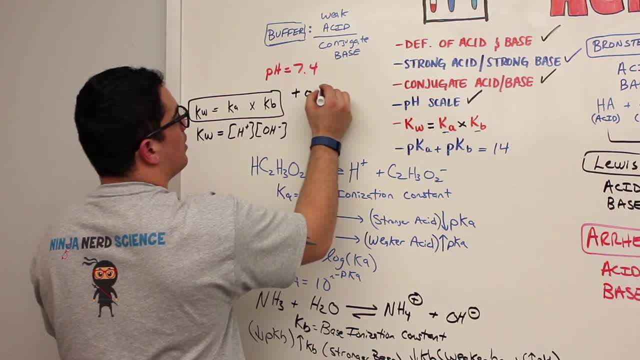 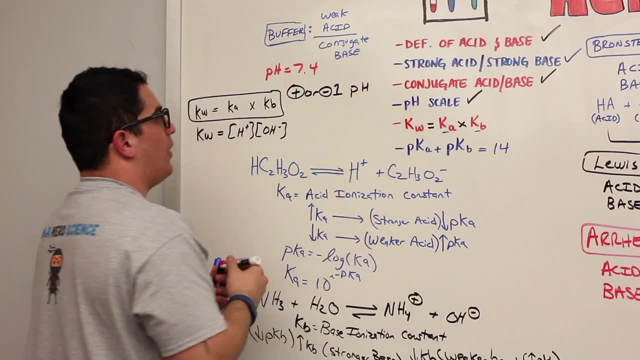 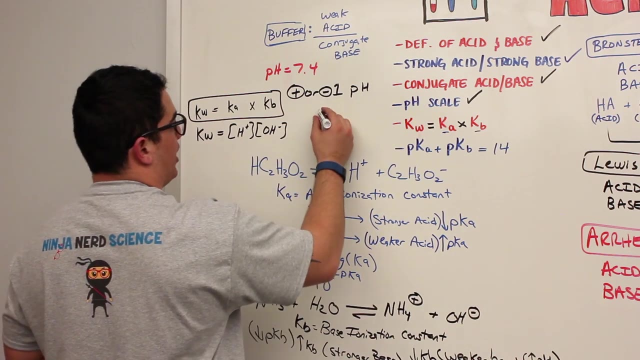 That's right. So the best buffer is plus or minus 1 of the pH. So anything that is plus or minus 1 of the pH is a good buffer. So, for example, if I had two buffers here, one of them had a Pka that is equal to 9.3,. 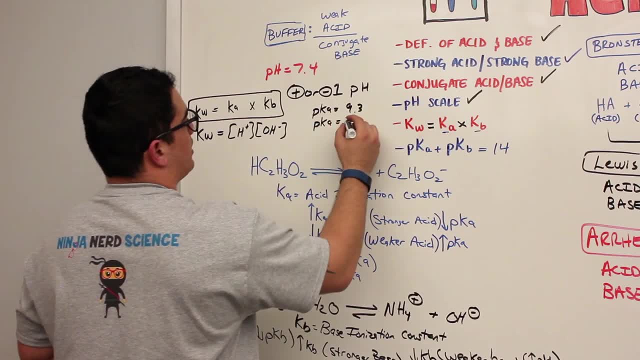 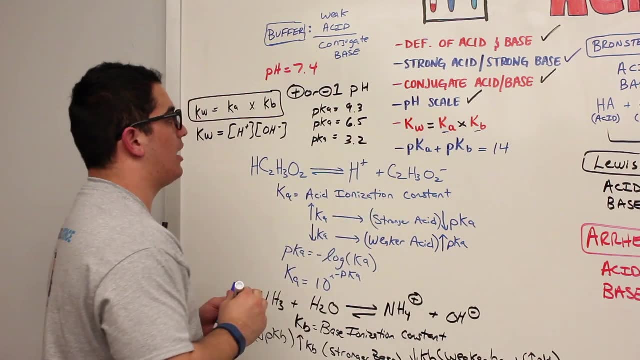 the other one had a Pka that's equal to, let's say, 6.5.. And I had another Pka that's equal to 3.2.. Which one of these am I gonna pick? I'm gonna pick the one. 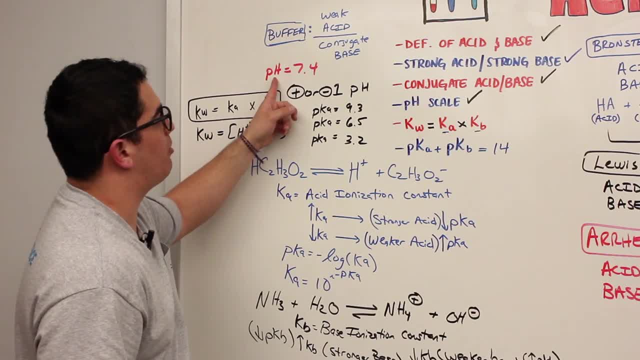 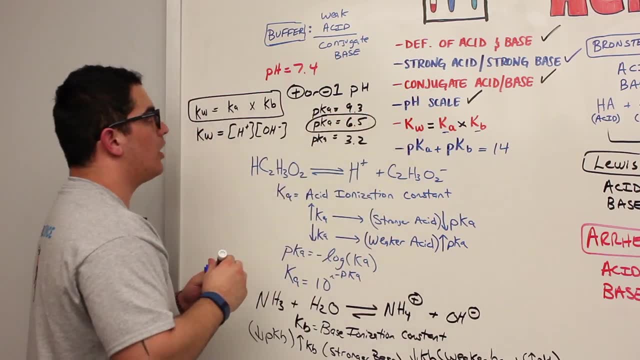 that's closest to the pH, because that's gonna give me the best buffer. Which one's plus or minus 1?? Oh, this guy right there, He's our best choice, So he's gonna be the best buffer in this case. Okay, so again, what have we talked about? We 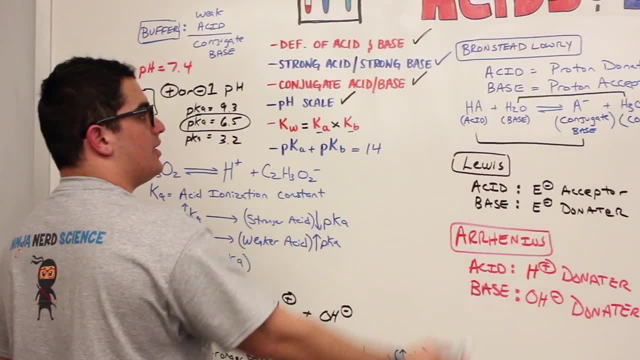 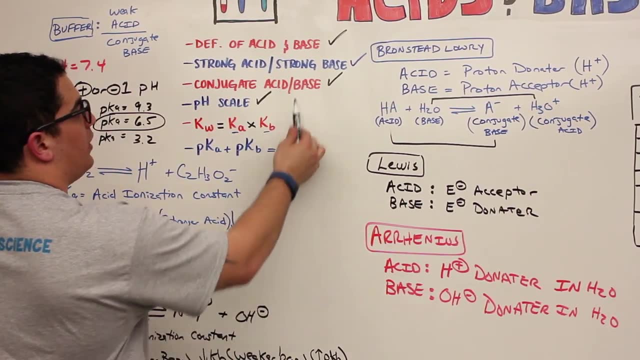 talked a lot, a lot of stuff in this video, guys. We talked about the definition of what an acid and a base is according to three different theories. We talked about all of our strong acids and strong bases and what that means to be a strong acid and strong base. We discussed conjugate acid-base pairs. We 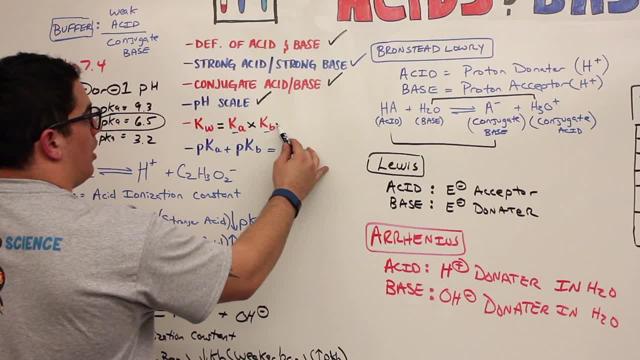 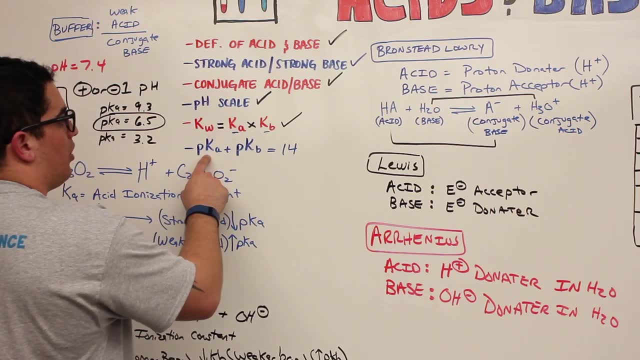 talked about the pH scale and its relationships and formulas. We talked about Kw- auto ionization of water- and Ka and Kb and their relationship to the pH scale, And then we talked about pKa and pKb with respect to buffers and also.